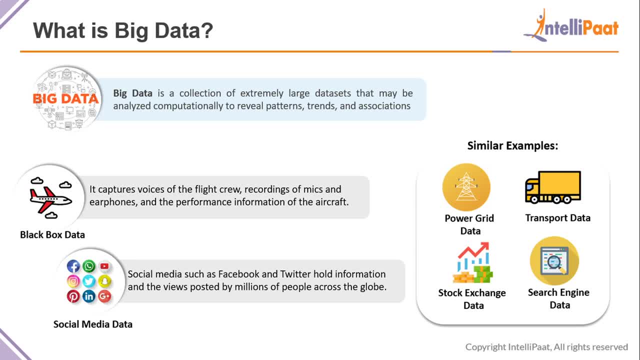 So, basically, whenever we have data in computational terms, we can analyze it to generate patterns, and such We can generate patterns, We can understand how that data progresses when certain variables are adjusted. So to understand the examples of what this Big Data means, 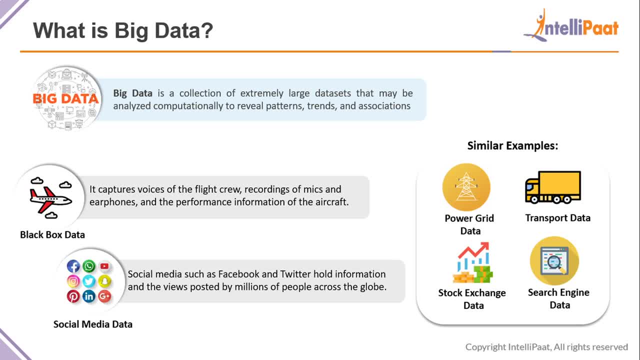 We can look at certain examples. Firstly, we have black box data, which means flight data, basically flight recorder data. Whenever there is a flight, it has a black box in it which captures the voices of the flight crew and the recordings of mics and earphones. 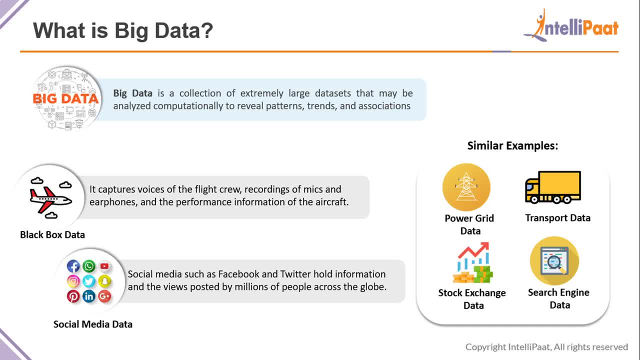 And basically the performance statistics of the aircraft. all of it is recorded and kept saved inside the flight. So in case of any mishap or in case of any investigations, the black box data can be investigated. And Since there are a lot of flights throughout the world in one day, we gather a large amount of black box data in the period of one day. 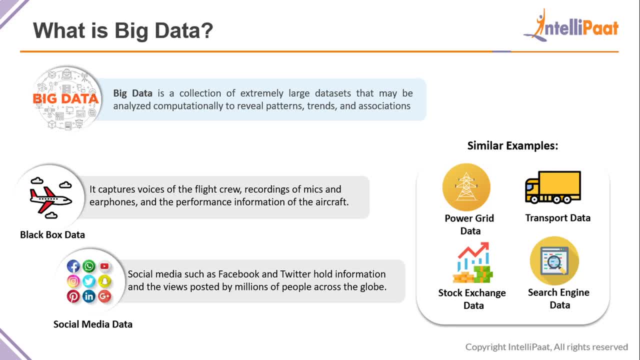 That is why black box data can be considered as Big Data. Then another very obvious example that we have is social media data. We all of us use social media in some form or the other. We use texting services, we use Facebook, we use YouTube. we use all of these. 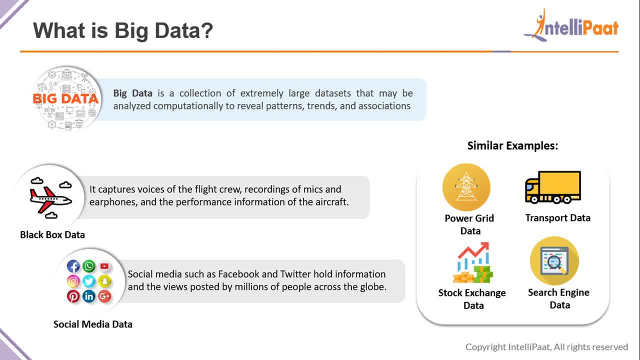 And we, all of us have accounts and all of us generate data as to what are patterns. And we, all of us have accounts and all of us generate data as to what are patterns. And we, all of us have accounts and all of us generate data as to what are patterns. 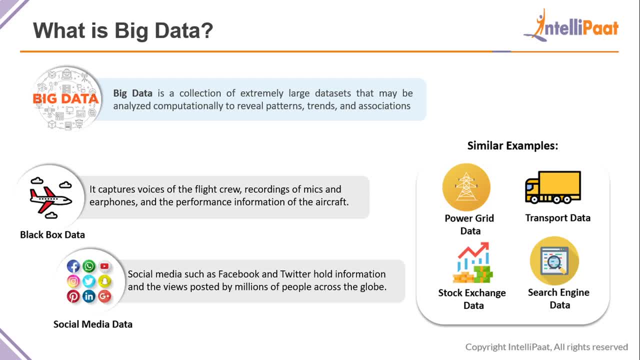 So don't be fooled: Every social media website basically stores every aspect of the data we generate on these websites, And to process and store these large amounts of data, we use Big Data analytics, And this sort of data can be termed as Big Data. 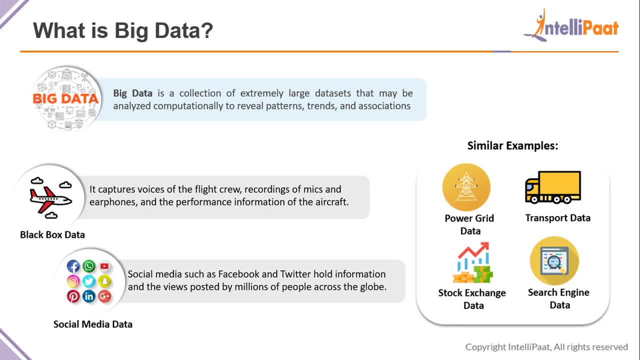 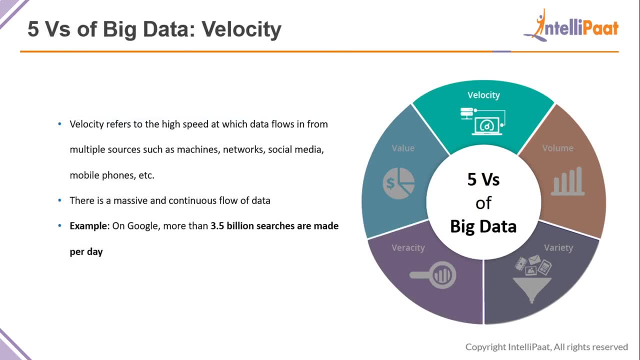 Other similar examples could be the power grid data, transport data, stock exchange data, you name it. All of it's there. So, moving on to the next, For any data or data set to be termed as Big Data, we need to fulfill five essential criteria, which are called the five Vs of Big Data. 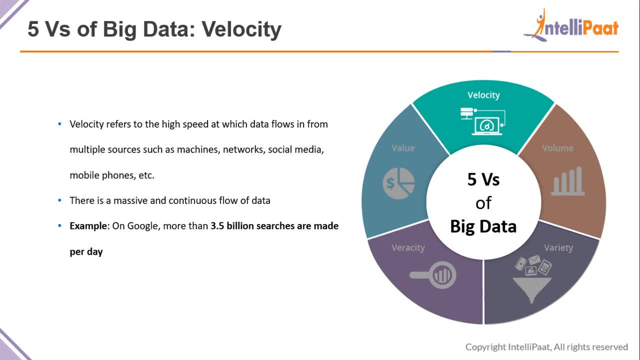 Because any data set over the size of one gigabyte can't be simply termed as Big Data, right. So there are five essential criteria for any data set to be considered Big Data. So first criteria is velocity. So velocity means speed. 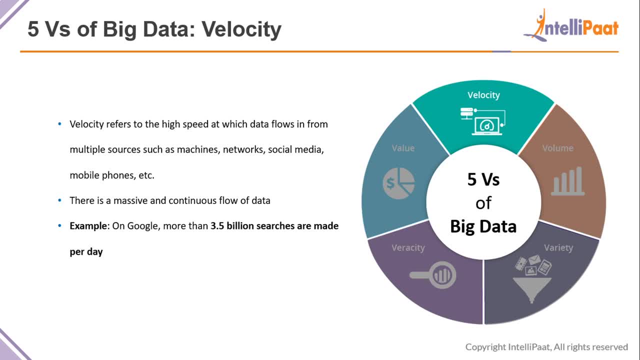 Obviously, if you've studied physics, you know what velocity means. It means speed. Speed essentially implies how fast the data flow is, how fast the data is being generated. If it fulfills a criteria- that the data is being generated really really fast- then it can be termed as Big Data. 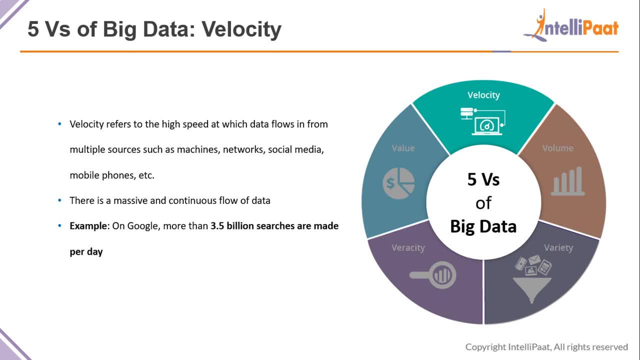 For instance, we have Google searches that are made per day. So in this example we have 3.5 billion searches are made per day. Can you imagine the amount of data that it generates? So basically, that means per day, the amount of data is really high that is being generated and it fulfills the category of velocity. 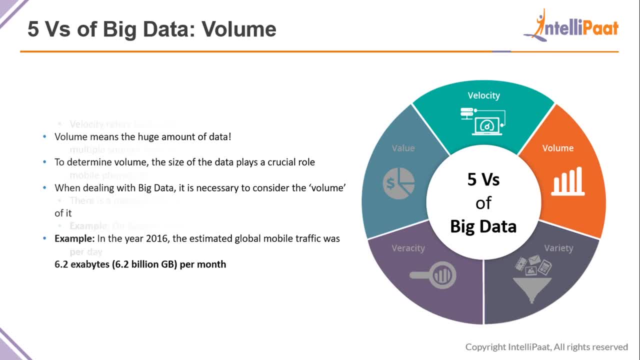 That is why it can be termed as Big Data. Moving on to the next V, we have volume. Volume essentially means size in the terms of computers And basically we have an example here for that 6.2 exabytes, which translates to 6.2 billion gigabytes per month of data is being generated in global mobile traffic. 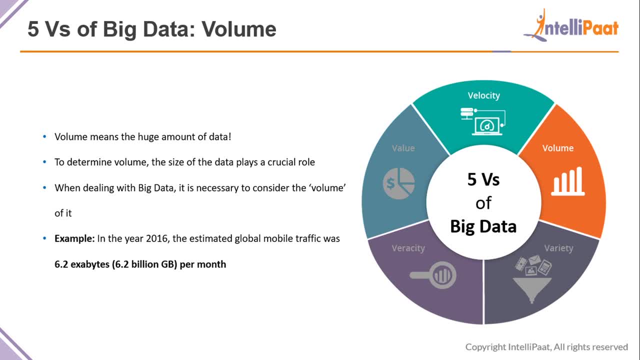 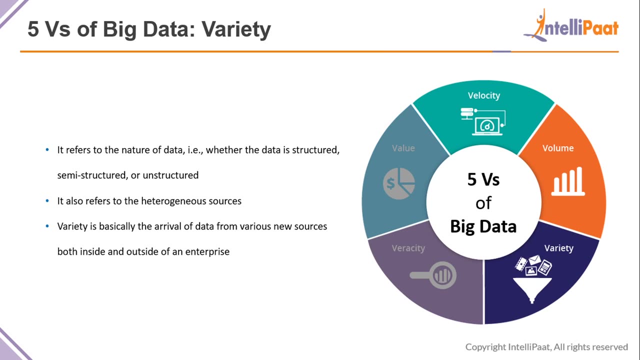 So that amount of data is really high and to process it would require non-standard tools, And that is why this sort of data would be considered Big Data, So volume should be high too. Next, we have variety, So there are essentially three sorts of data that is being generated right now in today's world. 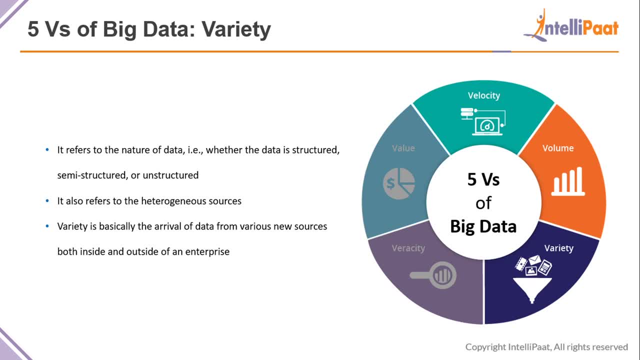 That is, structured, semi-structured and unstructured. Structured basically means that all the tuples, all the categories, all the variables, all the variables of the data are fully defined. The data is in an ordered format and it can be essentially processed the most easily. 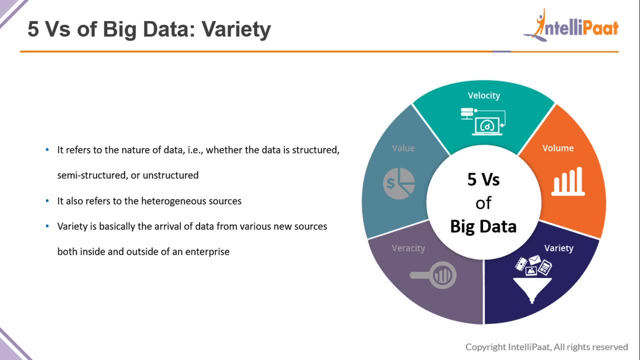 Structured data is the most easy to process. In fact, the process for processing unstructured data is converting it into structured first, and then we process it, And semi-structured is somewhere in the middle where it is sort of structured and sort of not structured. 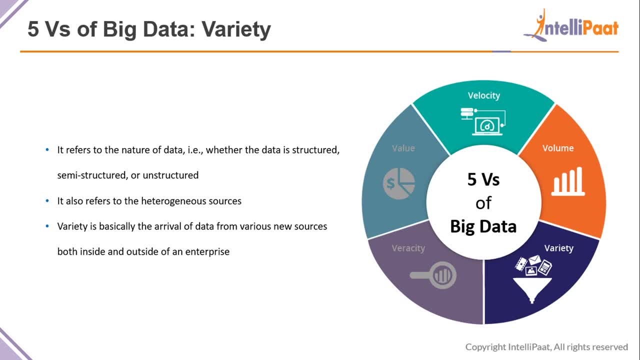 Some variables might be structured, some might not be, So it needs to have variety, essentially what it means. Next we move on to veracity. So the data can sometimes be inconsistent or messy is basically what veracity means. So Big Data isn't always perfect. 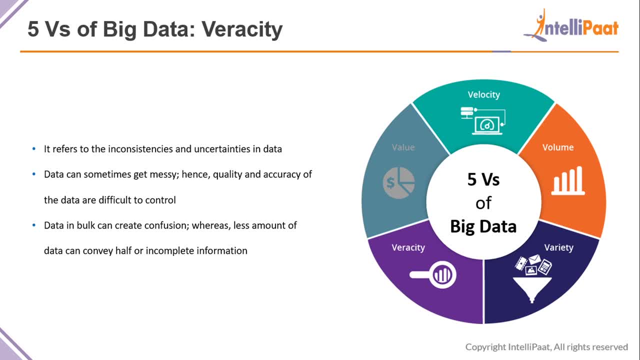 There can be certain inconsistencies in that data set And in real-world terms. when we talk about real data that is being generated out in the world, there's obviously veracity in it. There's no proper structuring to it. There's no proper formatting to it. 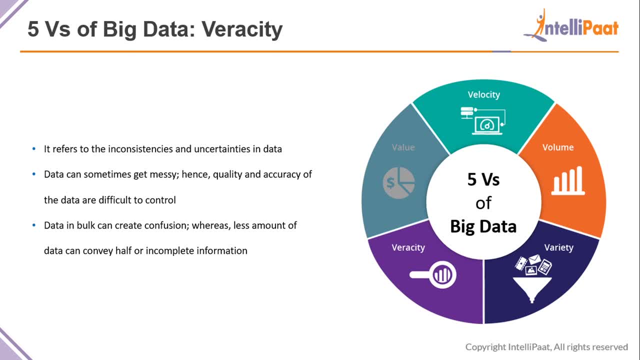 Then obviously there are a lot of inconsistencies in the real-world data that is being generated right now And that translates to veracity, And veracity is also a key factor in data being called Big Data. So then we have value. 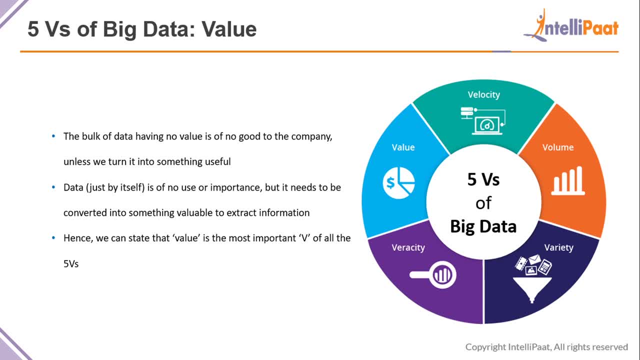 The value is the most essential V in the five Vs of the Big Data. Value means what and how much that data is worth. So basically, we can have bulk of data, but if it's useless, if it doesn't translate to anything, 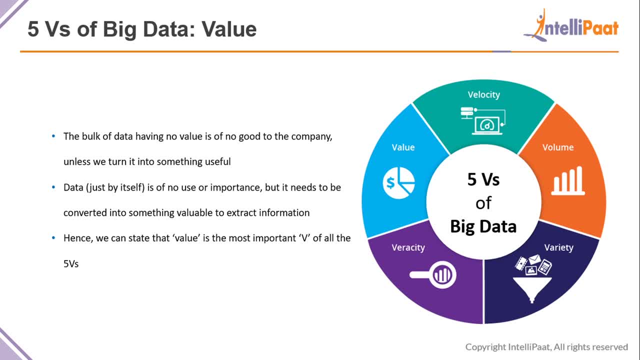 then all of that huge amounts of data would not amount to any good model, any good cost. So that's a computational analytical procedure. It doesn't make any sense. So basically say, for example, we have roll numbers in colleges. 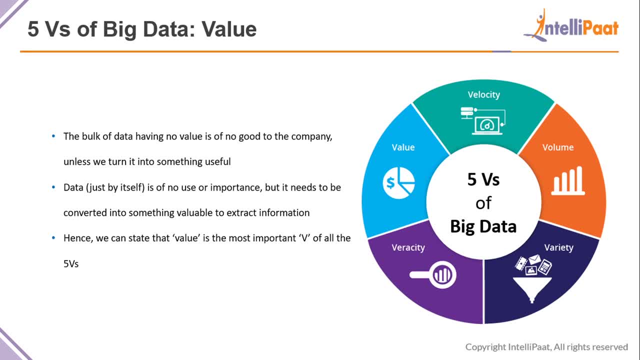 So if we take into consideration roll numbers- the primary keys of any table- the roll number doesn't equate to any model. It would not predict, It's not good for predicting anything, So that data we have to discard, So that data basically has less value as opposed to something else like marks. 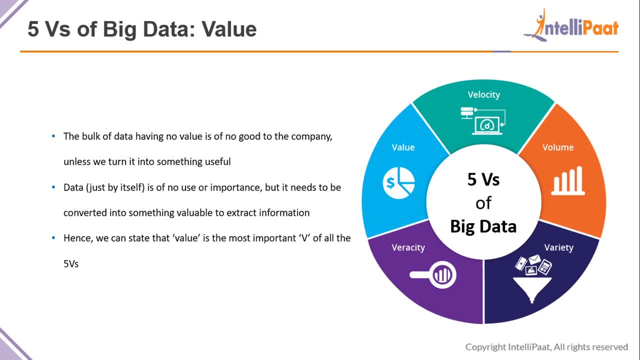 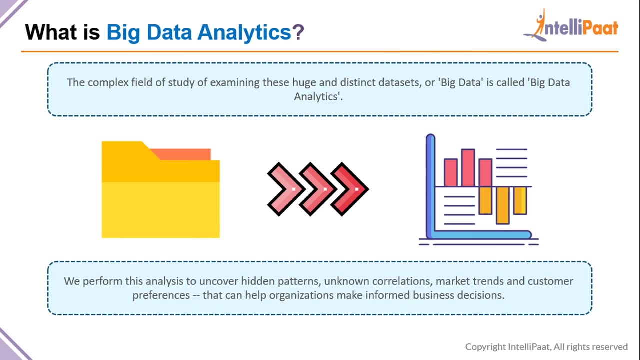 So this was essentially value translates to in the big Vs of data sets. So, moving on to the next, we move on to the definition of Big Data analytics. Now that we know what Big Data is, we understand what Big Data analytics is. 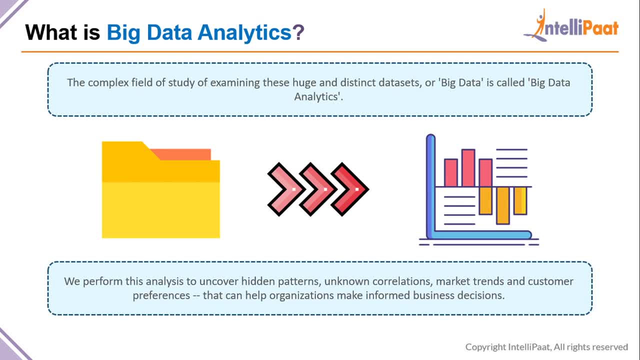 The complex field of study of examining these huge and distinct data sets that I discussed just now, or Big Data, is called Big Data analytics. So how do we process it? The entire study, the entire field of study related to that, is called Big Data analytics. 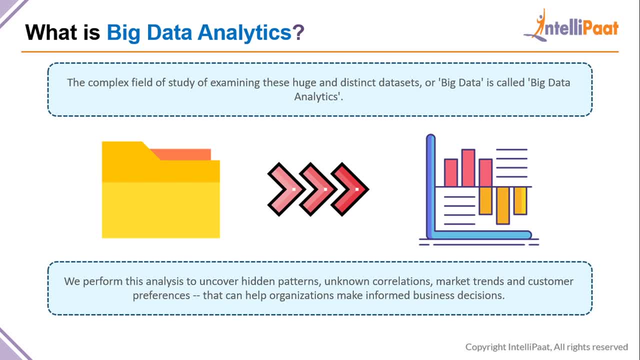 So why do we perform this analysis? This is to uncover any sort of patterns, market trends, customer preferences, Basically in business, we have a lot of websites, e-commerce websites. for them to understand what to recommend you, what to suggest to you. 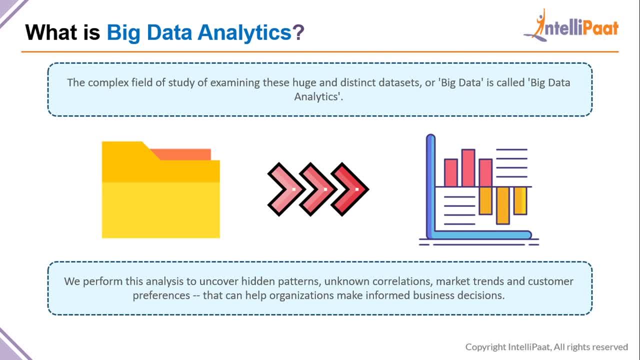 and how you behave on that website. It's very essential for them to process the data that you generate throughout your time on that website. So, basically, the art, the study related to uncovering this pattern from ambiguous data is basically Big Data analytics. 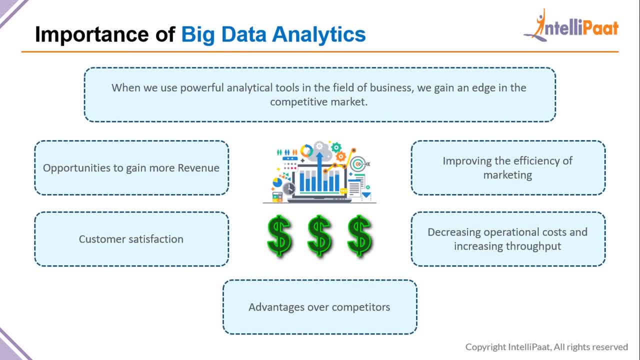 And the entire field of study is related to that. Moving on to the next, we have the importance of Big Data analytics. So we're going to be talking about the importance of Big Data analytics from a business point of view. basically, Businesses could be e-commerce, businesses, social media websites. 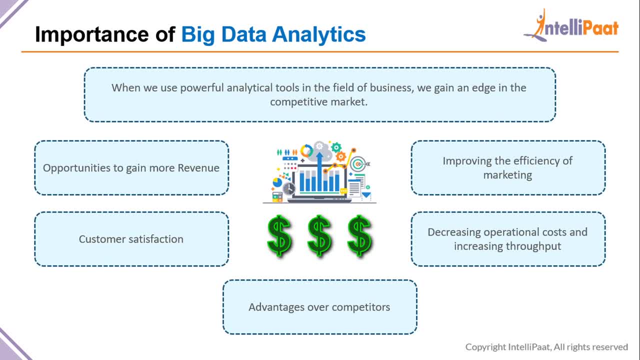 So social media websites also use ads. They use targeted ads towards you And when you click on those ads they earn money. So, basically, it's really important for them to understand what you do on that website to target those ads towards you. 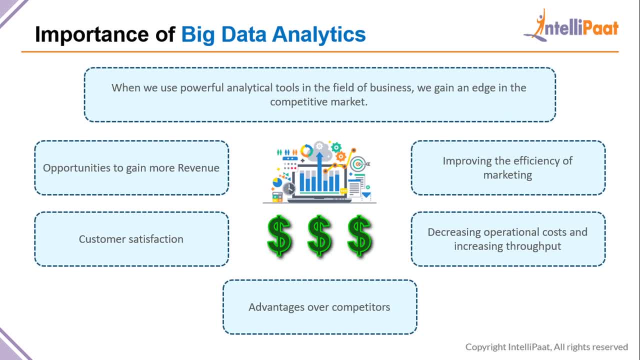 So we're going to be discussing five points here: Opportunities to gain more revenue. Obviously, everybody wants to make more money, So they need to understand what their consumer base wants, how their consumer base behaves. So that's why Big Data analytics gives them the opportunity for that. 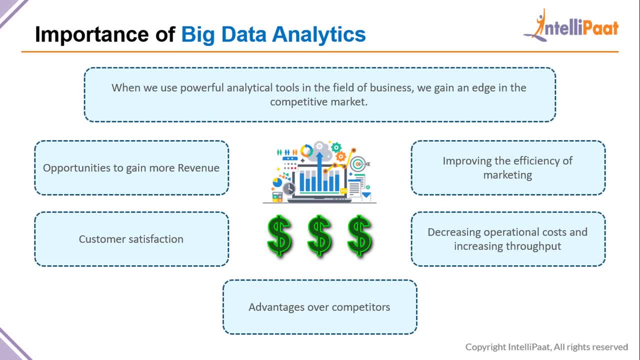 Customer satisfaction. If a website or service is oriented towards customer satisfaction, it obviously understands, by Big Data analytics, what the customer wants, So it caters to its customer's need and provides a fantastic service to its customer. That's why it fulfills the customer satisfaction criteria. 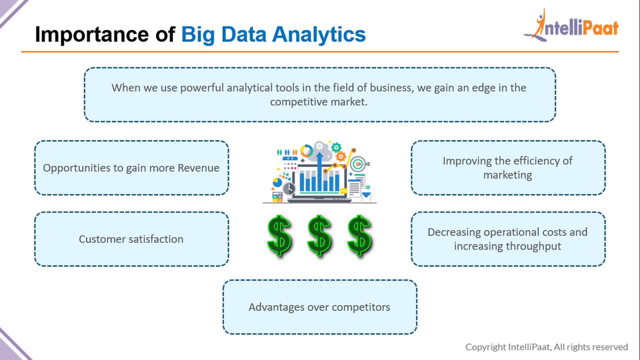 Advantages over competitors. Obviously, if a competitive website, a competitive business, is not using Big Data analytics, they don't have the edge over an organization that is using Big Data analytics. Traditional methods cannot do what Big Data analytics does, So basically, it gives them an edge over the competitors. 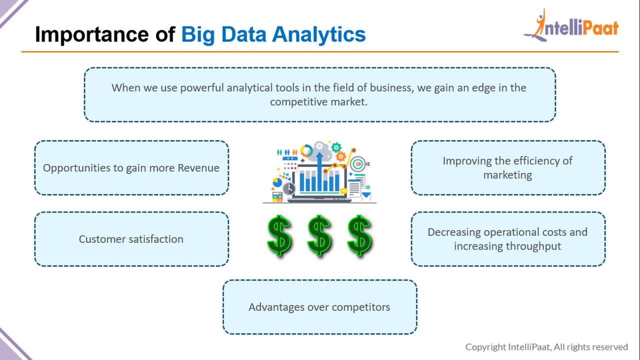 It depends on how good their algorithm is, how good they're processing their Big Data and how much value that their data has. Then we have improving the efficiency of marketing. So obviously marketing entails a lot of costs. If we target marketing towards a certain specific set of customers rather than blanketly putting an advertisement out there, 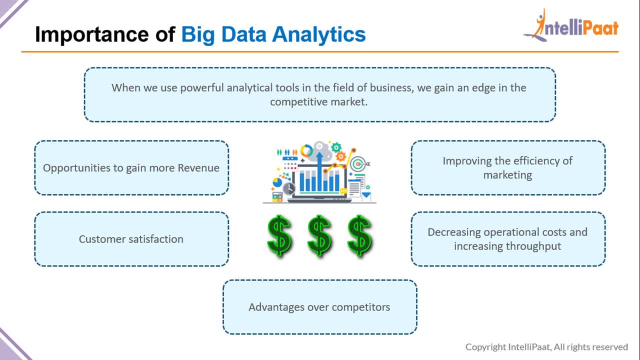 putting an advertisement out everywhere, then it obviously saves us a lot of money and increases the efficiency of marketing. This is something we can analyze using Big Data analytics: Decreasing operational costs and increasing throughput. So when we use computational methods to do things instead of manual methods to do it, we obviously have to do less work regarding it. 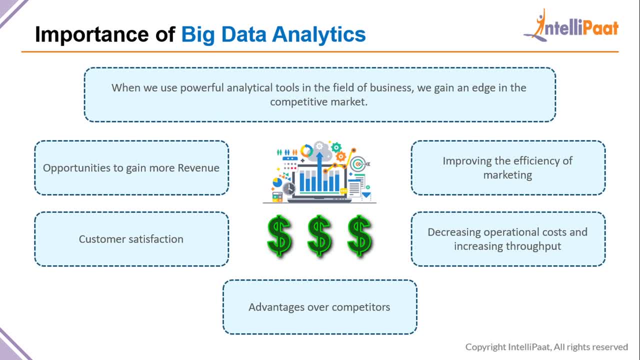 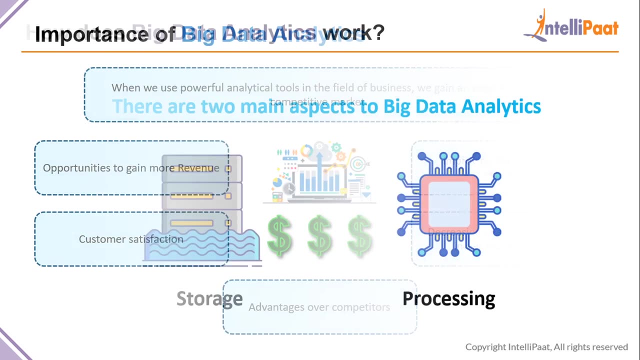 We have to do less research. The computer tells us everything, So the operational costs obviously decrease because we have greater information from Big Data analytics. So these are sort of the advantages and the importance of Big Data analytics. So moving on to the next. 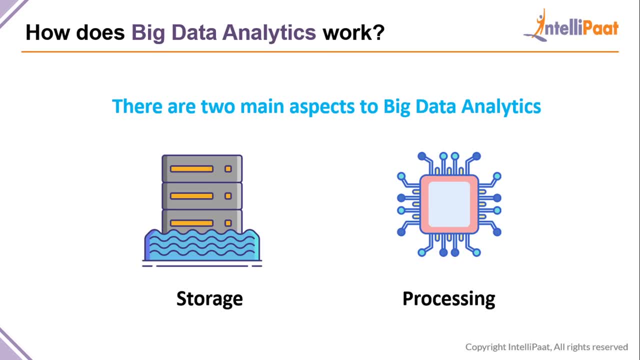 How does Big Data analytics actually work? So, in real-world perspective, there are only two facets to every sort of processing, every sort of computational activity in the world and the field of computer science. The first facet is storage, The other facet is processing. 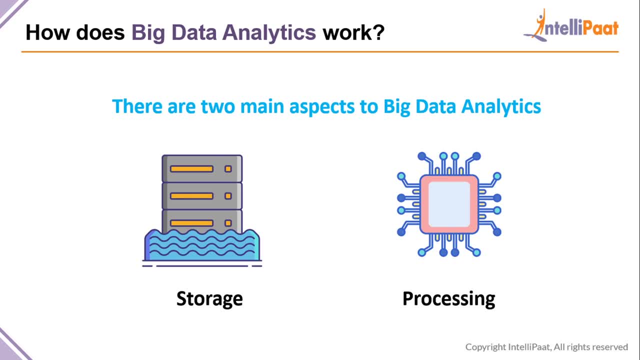 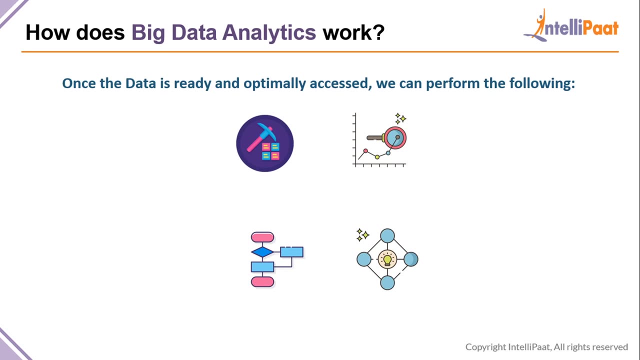 These are the only two facets in the computer science department where we need to spend money. we need to have good hardware resources to do these facets completely right. So what does this mean? So basically, once the data is ready and optimally accessed, when we perform Big Data, analytics on the Big Data and we put it in a sort of form where we can read it as structured form or semi-structured form, 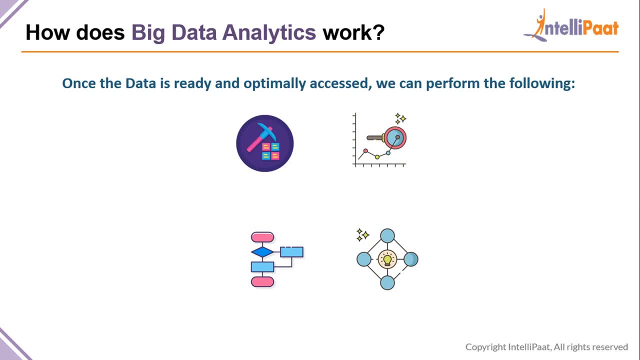 we can perform the following activities with it. That is where the analytics parts come in. So first is data mining. What data mining essentially means is taking a lot of information that might be ambiguous and turning it into something of meaning- Basically extracting data out of noise. That is what data mining means. 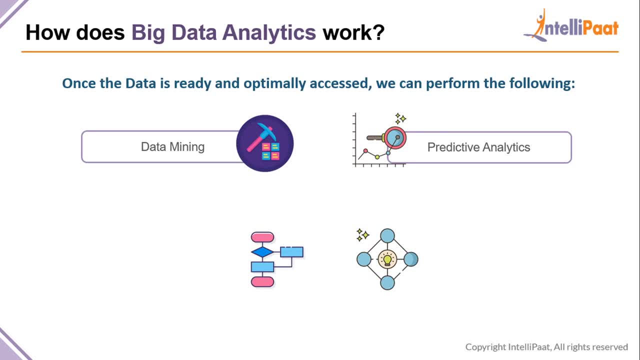 The next predictive analytics. Obviously, when we mined that data, we can perform analytics on it. We can create graphs and charts and predict Where data trends might go into. This correlates to the point I discussed before, which is understanding the hidden trends in data, which correlates to predictive analytics. 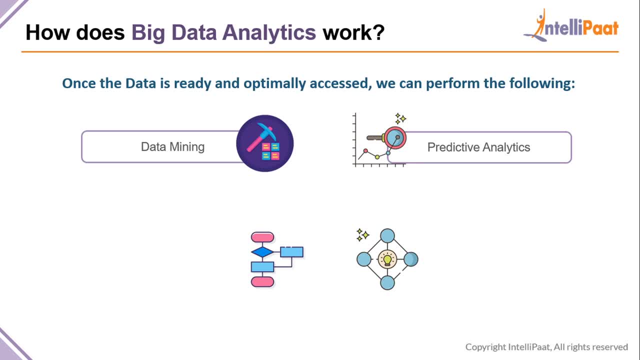 It's really important in the field of stock market businesses and understanding how sales might go when we alter certain variables and when we don't. Having a large amount of data gives a more accurate model. If you've studied machine learning, you would know the greater the training set is, the larger the training set is. 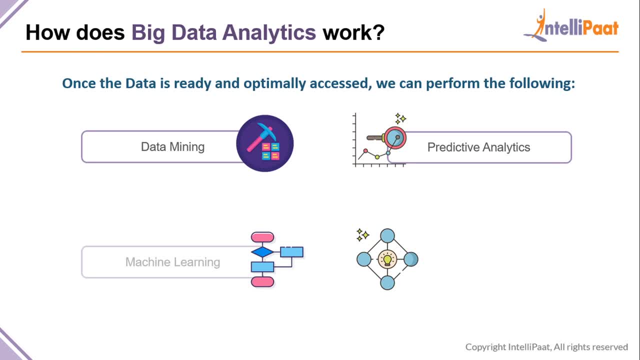 the better the analytics we can provide with it. Then we have machine learning, Obviously expanding on the predictive analytics part of things. we have another greater aspect to big data analytics, which is machine learning. Again, this correlates to the point where if the training data set is large- in this case big data analytics- it's extremely large. 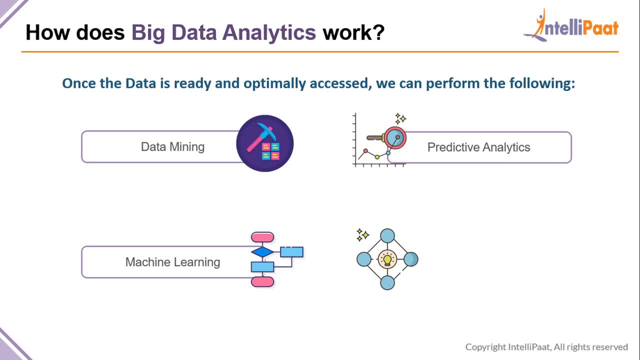 then the machine learning algorithms. the machine learning models that we would create from those algorithms would be more and more accurate As the size of the data increases. Then, expanding on machine learning, we have deep learning. Machine learnings are basically simple models and deep learning are convoluted neural networks. 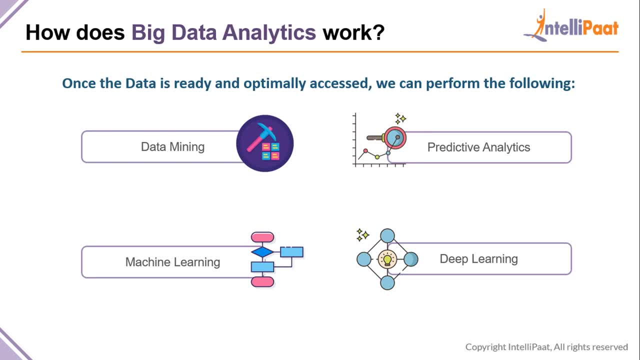 If you studied machine learning, you would understand what deep learning is. It's to create more complex models with a higher number of constraints and variables, Having basically all of this equates to the more data we have, the better model we have, The more models we can create and the more value of those data it would correspond to even better models. 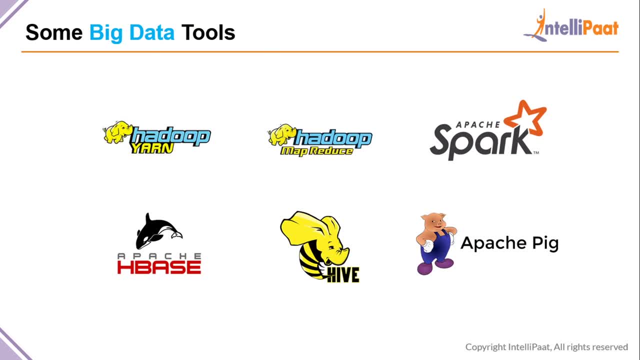 Moving on to the next thing, that we have some big data tools that we have. If you've been doing big data courses or if you've been looking up tutorials, you would know all of these tools. You might have heard about them. The first is Hadoop YARN, obviously the resource manager of Hadoop. 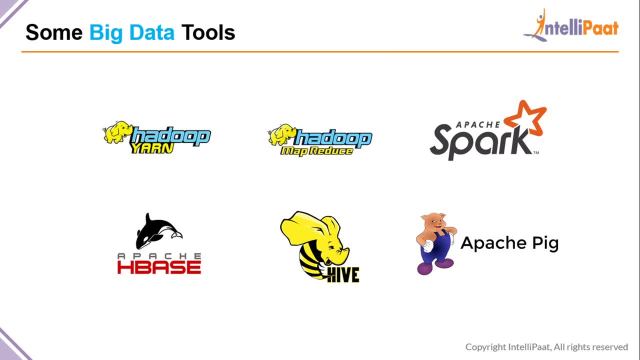 Hadoop is a software that we use for big data. essentially, YARN manages the resources that we allocate to jobs and such. We have MapReduce, which is the actual, the main thing that Hadoop has. It maps data and then it reduces it. 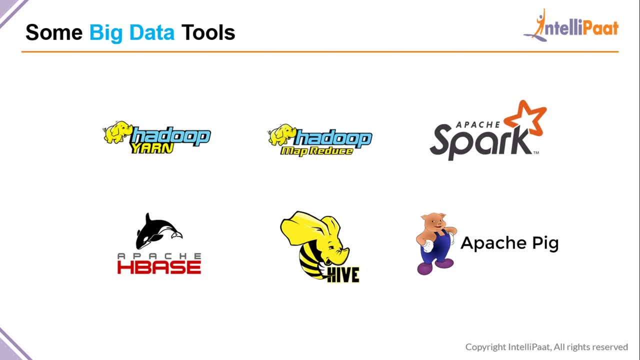 It maps data into certain parts and then it's sent to the producer. The producer aggregates the data. That is the model that Hadoop follows. Essentially, all of big data today is processed in clustered forms. We have tons of nodes spread across. 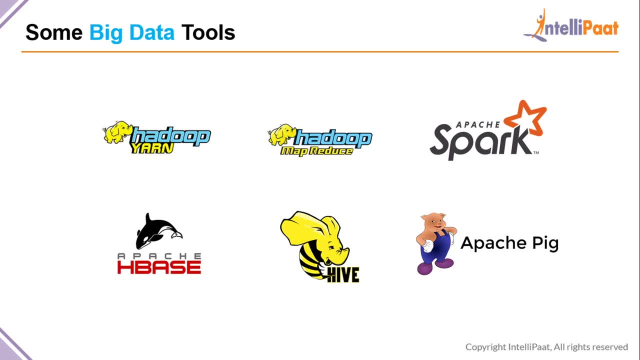 Commodity level hardware that is easier to afford than, say, advanced level hardware that was used previously to process big data. Today we use commodity level hardware with the use of cluster management, Hadoop and Spark and all of these softwares that are being used today for big data use the cluster node- sort of logic. 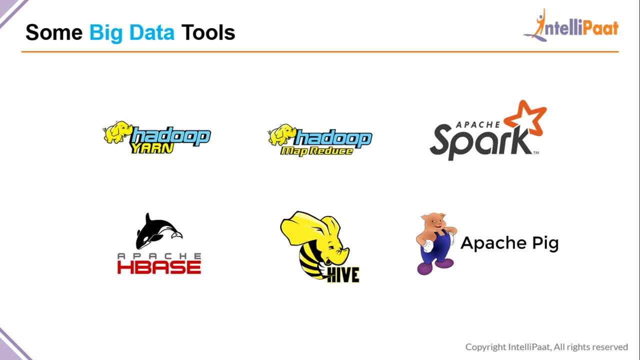 Then we have Apache Spark, obviously what we're going to be discussing about today. Apache Spark also helps in processing of data In a much more faster manner than Hadoop, although it uses Hadoop as a base for things, as a storage criteria for things. 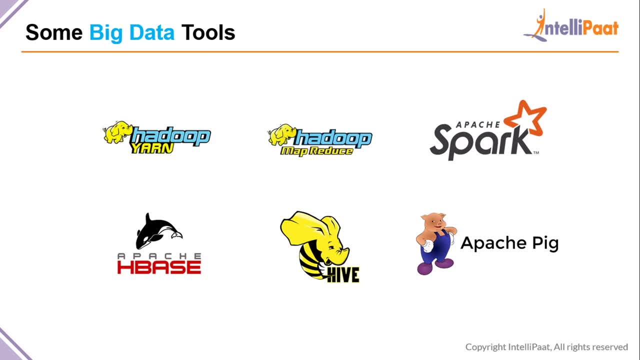 But Spark expands upon Hadoop by performing much faster ways to implement MapReduce operations or Hadoop big data operations. essentially, We have HBS, We have Hive. Hive essentially implies not changing the actual data but giving us the view of that data and processing it from the above without actually altering anything inside the HBS. 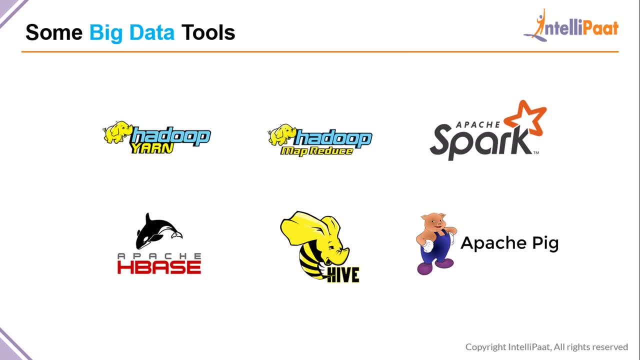 It basically takes the view of the data, performs some operations on it, gives you the output, but doesn't actually change the actual data. We have PIG for large amounts of web logs that are created from websites every day. To process those large amounts of web logs we use Apache PIG. 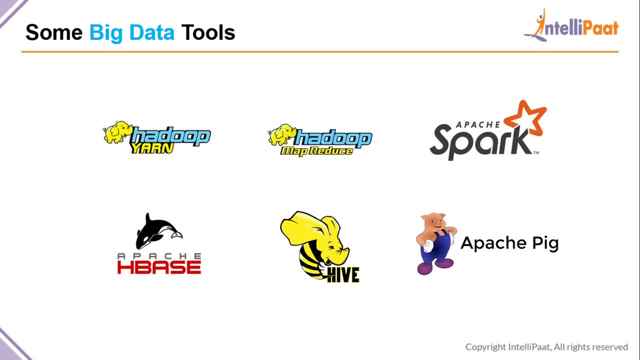 These are some of the tools that we use generally for big data and big industries. So we're going to be talking about Apache Spark today and how to implement Apache Spark with a hands-on approach. So we move on to the next topic, which is Apache Spark, obviously. 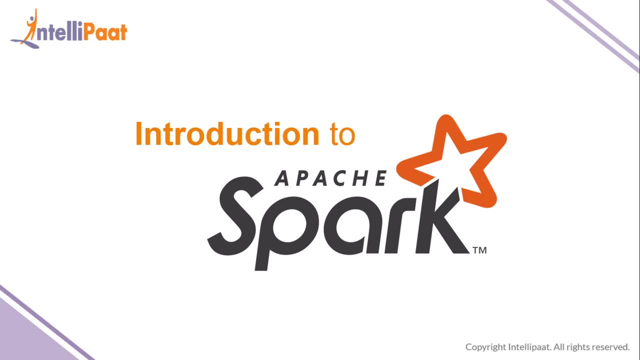 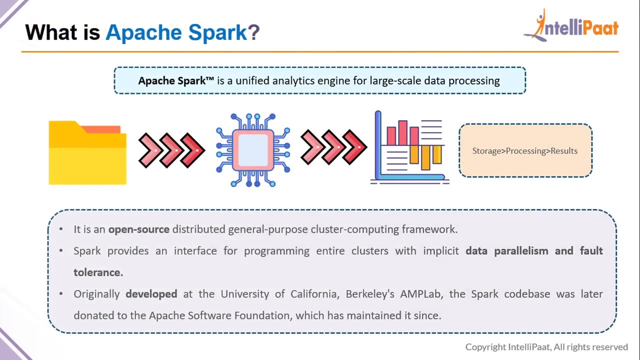 So, talking about Apache Spark, it's a framework provided for Hadoop, So what it essentially does is provides, as we can see, a unified analytics engine for large-scale data processing. So it takes up files from the storage, processes it and gives us the results. 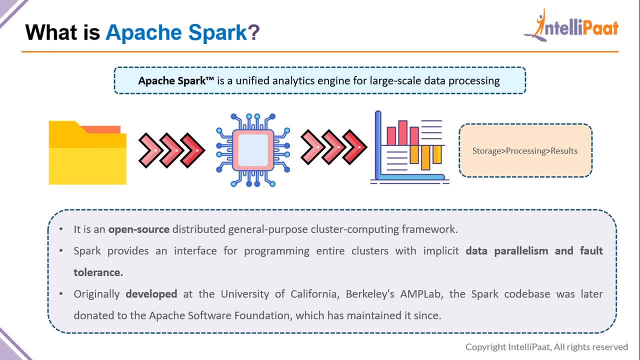 So it's open source, so it's easier to understand, It's easier to alter according to your needs because it's present in an open source environment. So the advantage of Hadoop, the advantage of Spark, essentially, is it provides an interface for programming entire clusters with implicit data parallelism and fault tolerance. 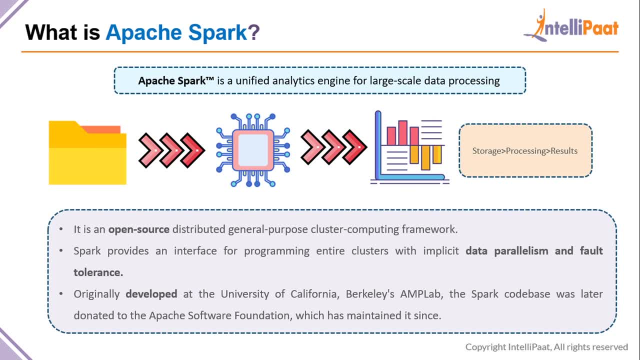 Which means even if you lose data on one node, even if you process data and it somehow gets into a fault, you can re-access the data because it's a cluster-based management system, So it basically replicates itself all across the nodes and you can access it from another node. 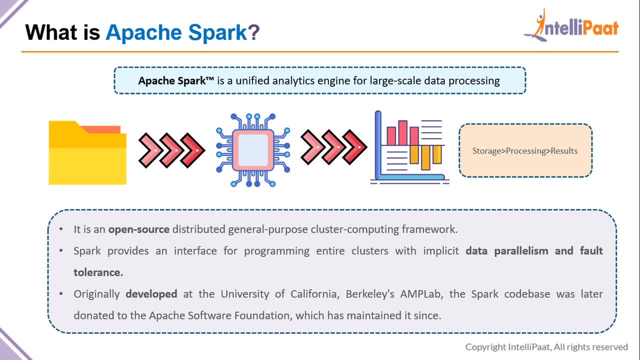 And data parallelism implies that when you process the data it happens in parallel on different nodes, so it's done faster. And a little bit of background history on Spark. It was originally developed at the University of California, Berkeley's AMP lab. 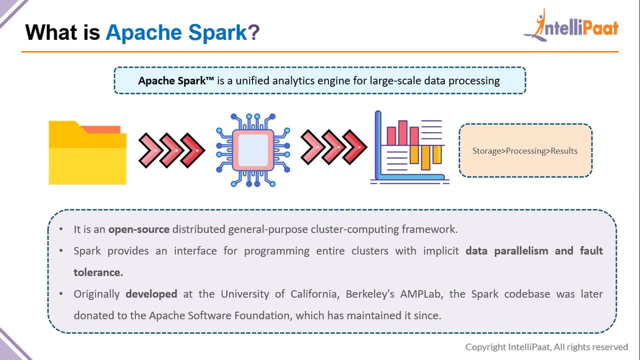 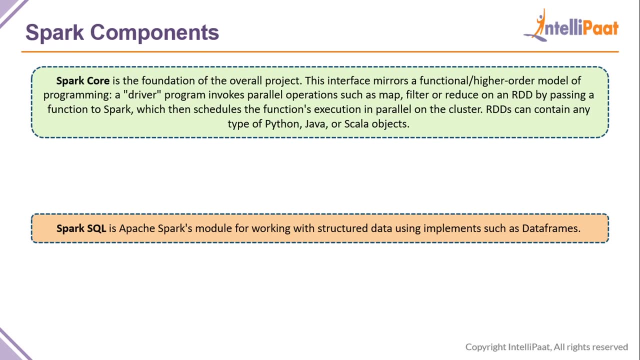 The Spark code base was later donated to the Apache Software Foundation. We're talking about Apache Spark today. It was developed as an open source software at the University of California and then it was donated to Apache Software Foundation. So, moving on to the next, we have Spark components. 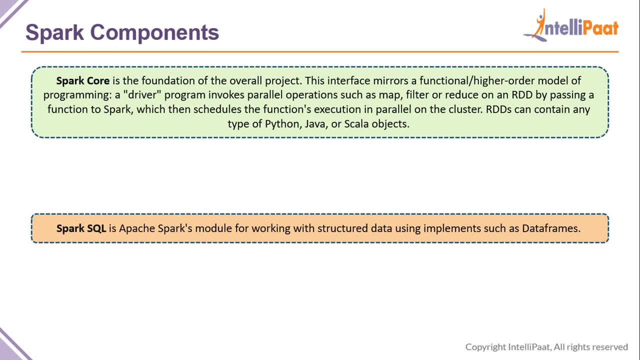 The Spark core, the main component that Spark has, which essentially correlates to the RDDs, the main thing about Spark, the main advantage about Spark. So what are RDDs? So RDDs are resilient RDDs. So RDDs are resilient distributed data set. 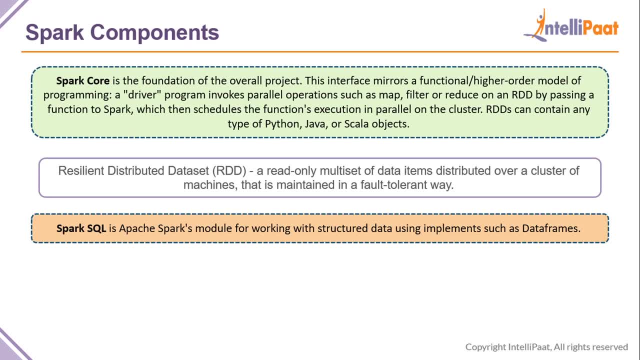 A read-only multi-set of data items distributed over a cluster of machines that is maintained in a fault-tolerant way. Again, the aspect of Spark is fault tolerance, which means data replication. If a fault occurs at any time of the processing or the execution of a Spark operation, the data is replicated and we can access it again. 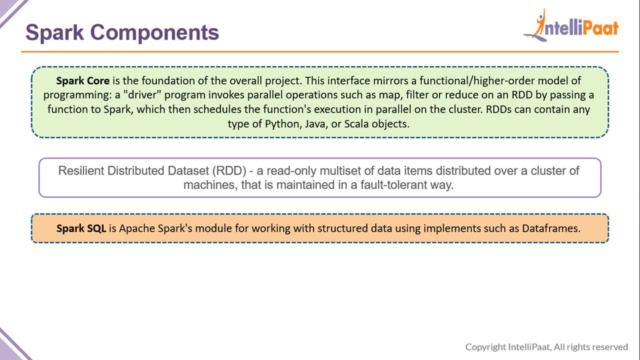 And an RDD essentially means that when you create an RDD it might be a huge RDD, So that's a big thing considering on the amount of data that you've inputted into that RDD. So to manage that large amount of storage, an RDD can spread itself across various nodes. 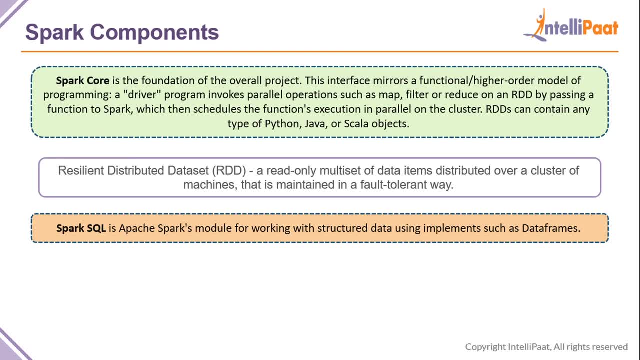 And that is what cluster-based management in Spark basically means. That is what an RDD is. So an RDD can be implemented in many ways, That is, via Python, Java or Scala objects, as you can see, And then we have Spark SQL. 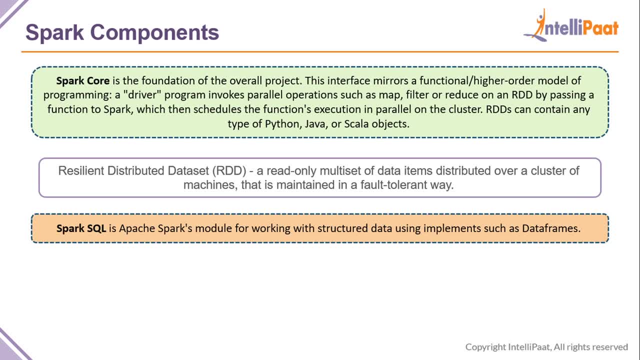 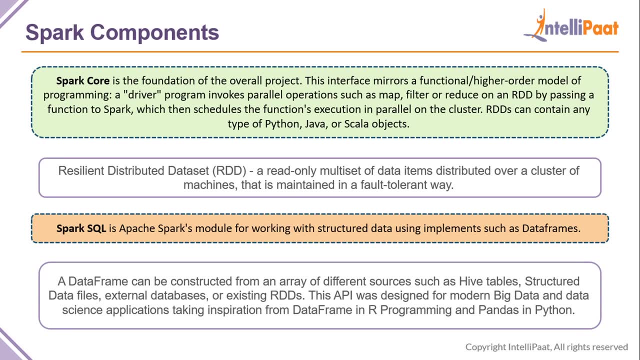 Of course the facet of Spark that lets us deal with the relational database management system implements. So Spark SQL expands upon RDDs with providing us data frames. So data frame is essentially an extension of an RDD where we can use sources such as hive tables, structured data files, CSV files or external databases or existing RDDs. 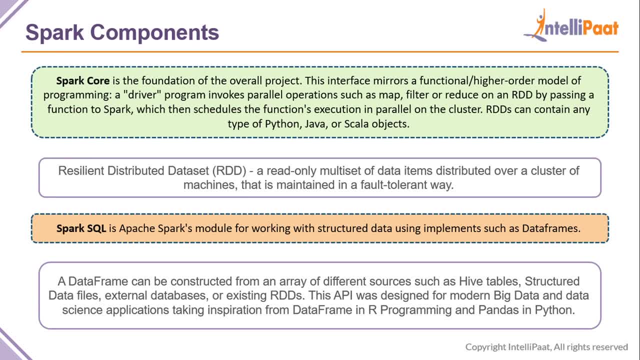 We can also make data frames out of existing RDDs. You would know what data frames are if you've done Python machine learning or machine learning with R. It's sort of based on the same logic And, as you can see, the inspiration has been there. 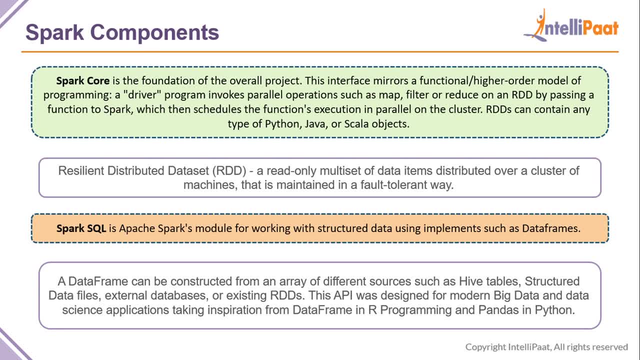 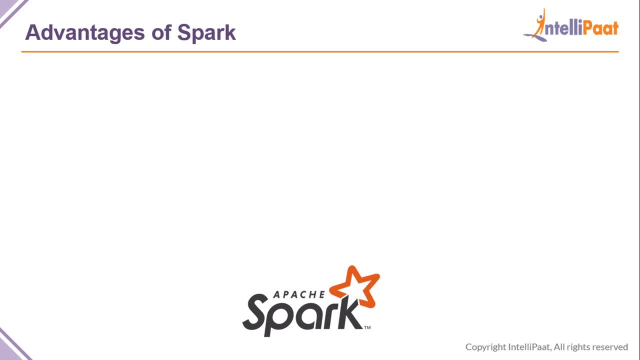 So, now that we've discussed what Spark components are, we will now discuss the advantages of Spark over traditional Hadoop operations, Hadoop processing operations, Hadoop methodologies. The first is speed. Obviously, the reason we would replace a pre-existing procedure with anything new is because it's more efficient. 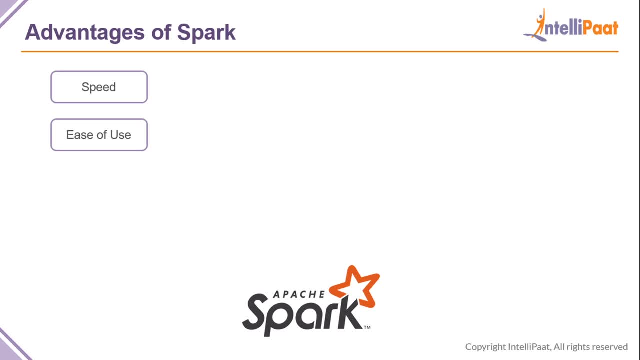 So the first is speed. Then we have ease of use. Obviously, Spark is much more easier to use. Hadoop provides us a lot of things with legacy-level implements and it's harder to understand for newcomers and harder to understand when you're learning something from the start. 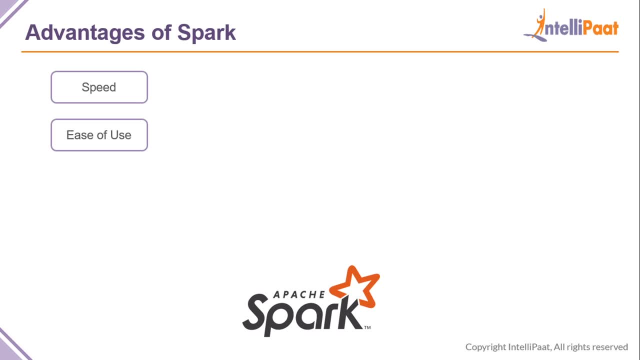 Obviously, Spark provides us with an abstraction over Hadoop. It's easier to use. Then we have generality, Then we have a runs-anywhere sort of implement. So basically, Apache Spark is almost platform-independent. So it runs workloads 100 times faster. 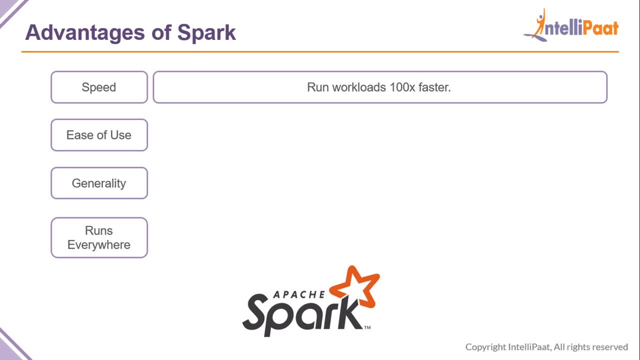 100 times faster in this case would imply that it runs 100 times faster compared to Hadoop- legacy Hadoop. Then we have ease of use. We can write applications by not going into legacy coding methods. We can use Spark using Java, Scala, Python. 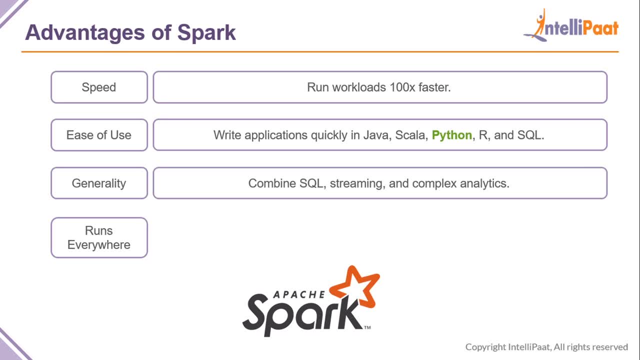 We can use Python, R and SQL. Then we have generality, Combine SQL, streaming and complex analytics. It basically gives us the option to combine all of these rather than having three separate terminals for all of these three, Three separate APIs for all of these three. 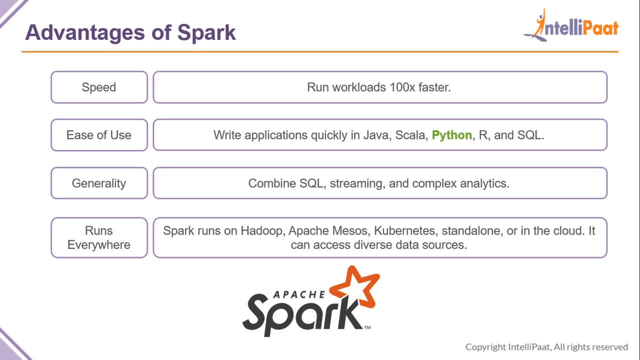 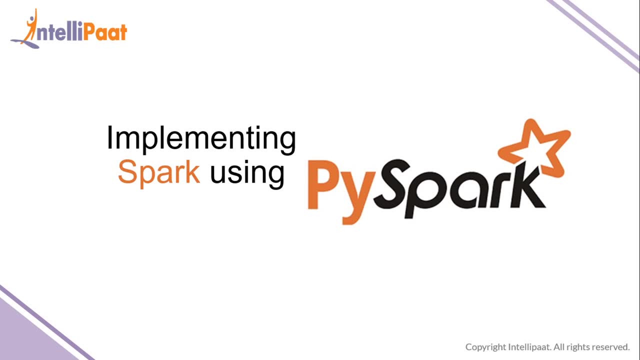 Runs-anywhere. Spark runs on Hadoop, Apache, Mesos, Kubernetes, standalone or in the cloud. It can access diverse data sources, So that is pretty much self-explanatory Implementing Spark using PySpark. So basically, we've discussed what Apache Spark is. 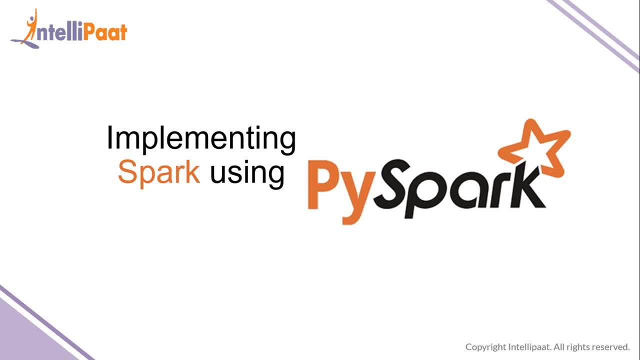 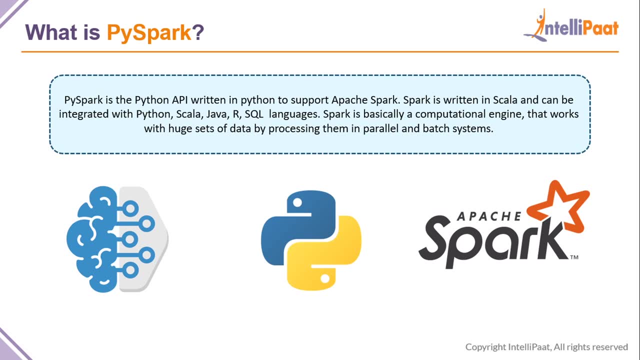 Now that we can move on to implementing it with a bit of hands-on. So firstly we will discuss what PySpark is before we move on to the hands-on guys. PySpark is the Python API, So it basically is: the Python gives us an API to write Spark code. 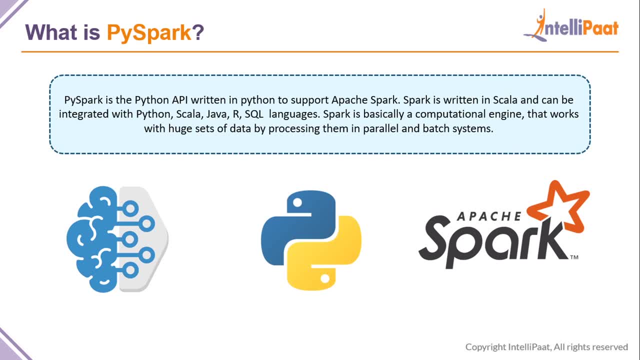 So, rather than writing Spark in Spark terminal, we can write it in Python and it will do the exact same thing. In fact, give us better opportunities and better methodologies, Because Python obviously supports machine learning. And if we were to implement and integrate both of these two- the advantages of Python and Spark? 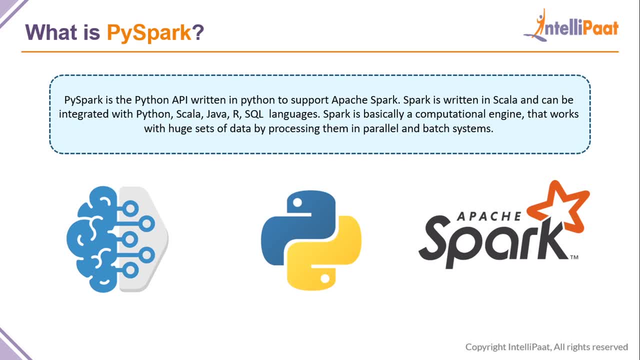 and put it into one platform, rather than driving ourselves crazy with implementing it on two platforms. we can use the PySpark API that is provided by Python. So basically, Spark is a computational engine which processes things, And if we are using PySpark, 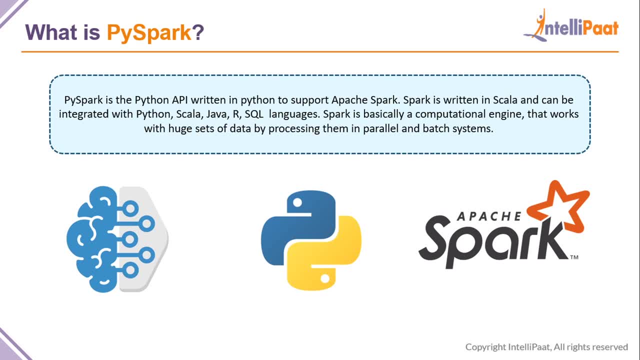 what basically Spark does is: Spark does the processing part of it and the storage part of it, while Python does the commands, the execution part of it. So executing and storing things on a cluster management system is done by Spark, while Python just is used to write commands. 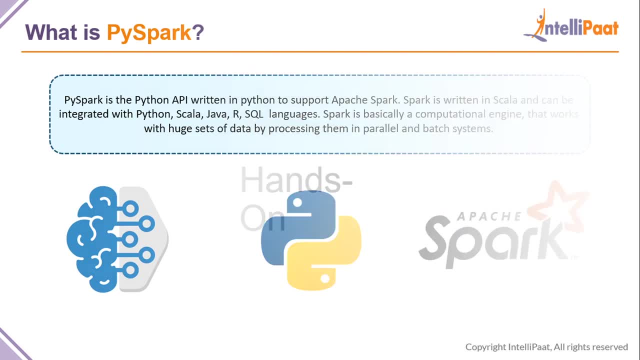 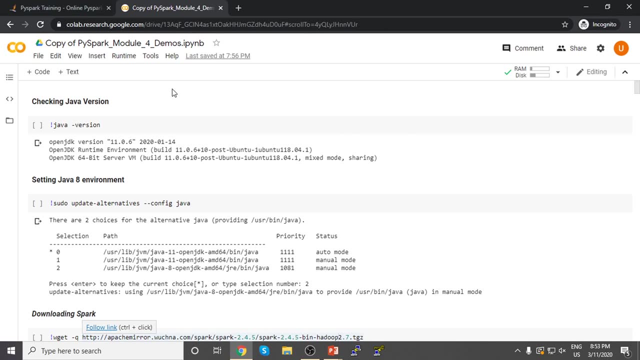 So, moving on to the next, we move on to the hands-on. So we have collabresearchgooglecom. This is basically a Jupyter notebook that we use. So rather than starting a virtual machine or starting an AWS instance, which would require lots of money or processing power on your PC, 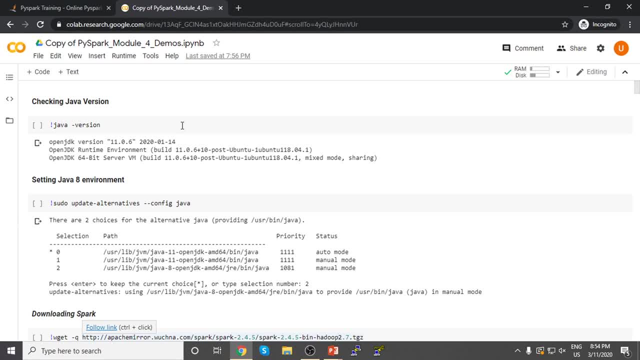 we could just use the collabresearchgooglecom, that Jupyter notebook implement that Google provides, So we can run it essentially as a Linux terminal, And that is what I've been doing here. So, firstly, what you will have to do is: 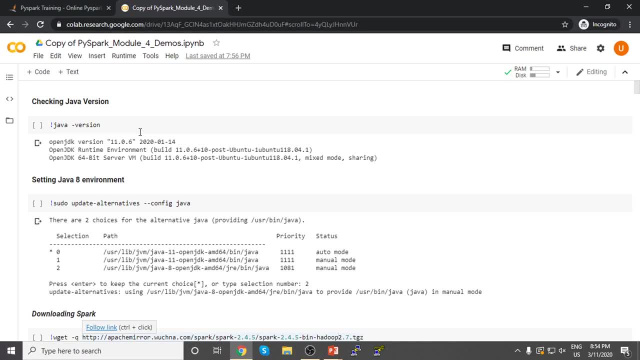 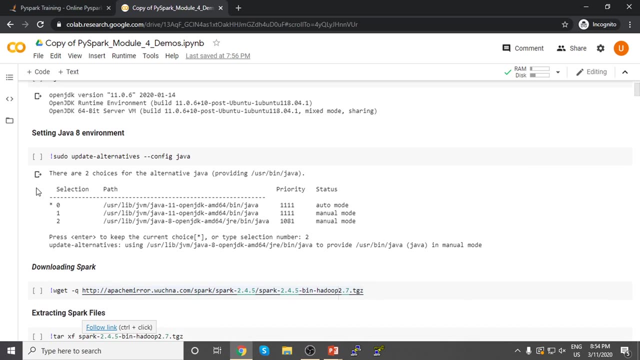 check what Java version that your terminal, that your Jupyter notebook Linux implement has. So first we'll check that with the Java dash version. So, as you can see, we have 11.0.6.. So to basically implement Spark, we need Java 8 to run it in the most efficient manner possible. 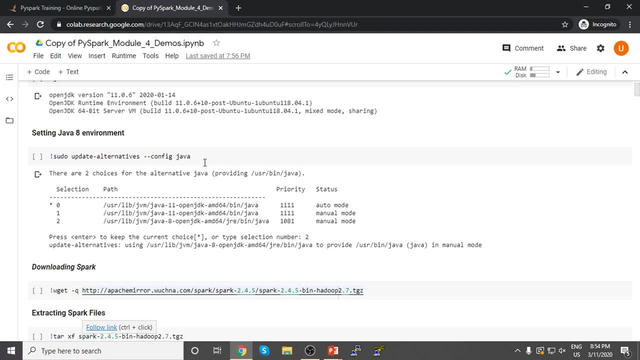 So we'll do a sudo update alternatives config Java. Then we'll get three options and we'll select the manual mode, because we want to set the environment directories according to our own. If we set it on auto mode, then it will set it on its own. 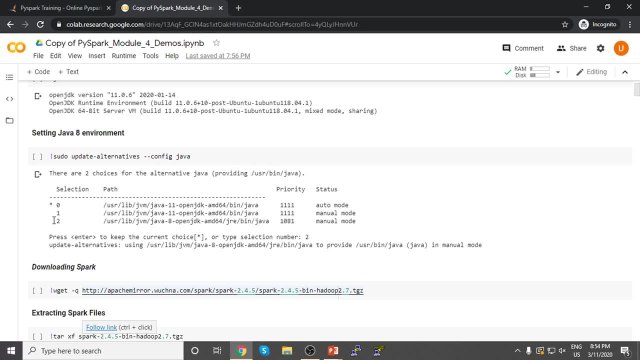 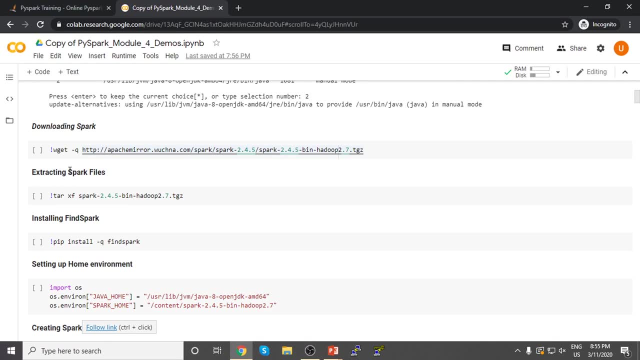 But right now we want to do it manually, So we'll input two. We will move on to the link that we have, The current link, the updated link. we have to download Spark 2.4.5.. We'll do a wget which basically gets it from the website. 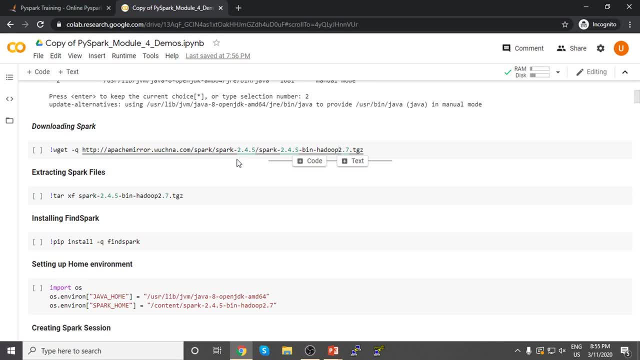 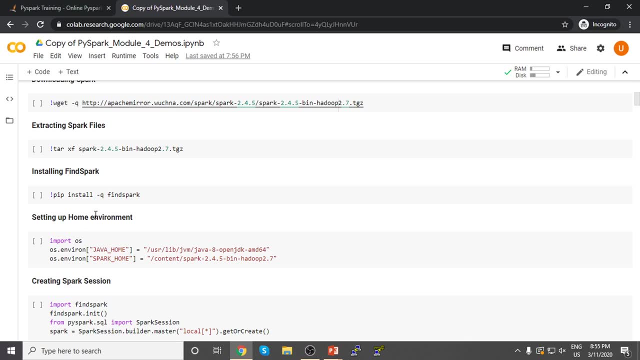 from the Spark servers that we have, the Apache servers that we have. Then we'll extract the compressed file that we'll get. We'll install find Spark. If you know what find Spark is, it basically helps us to helps the Python implement to understand where the Spark is located on the PC. 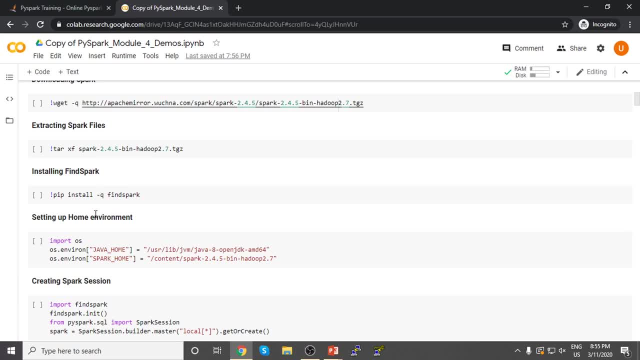 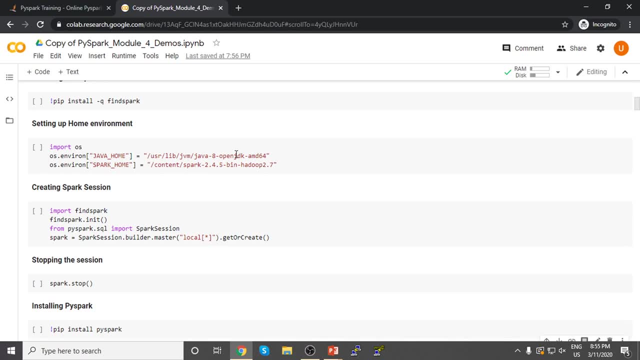 And then we'll set up the home environments for both Java and Spark. Since it's a manual setup for Java, we'll obviously do an OS dot environment and we'll put in the address for Java. Then we have Spark home And where Spark is installed we'll provide that address. 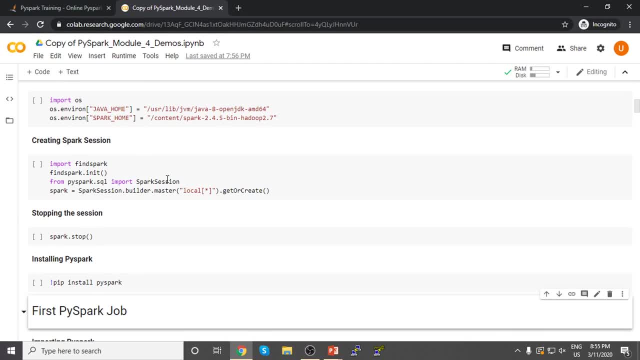 So, firstly, we'll start by seeing how a Spark session is created. We import the find Spark, which helps us see this is Python code. right, You can recognize this is Python code. So, basically, the find Spark helps us to understand where the Spark libraries are located for Python. 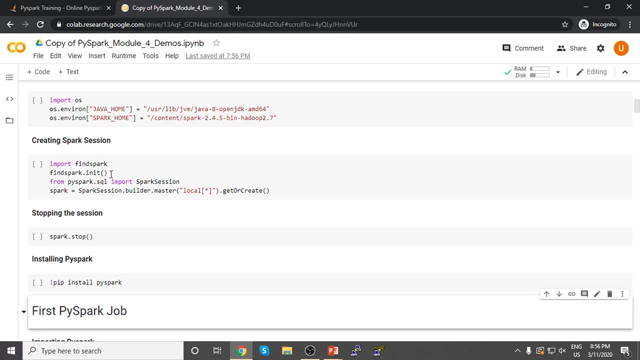 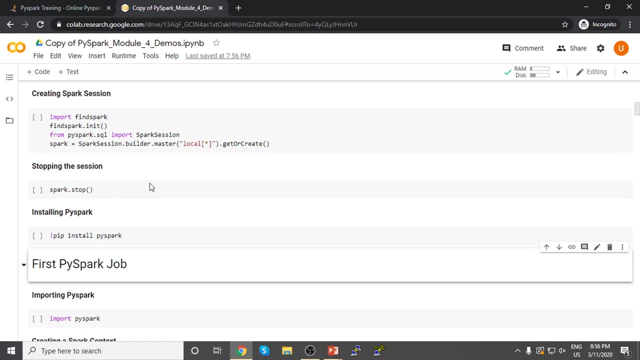 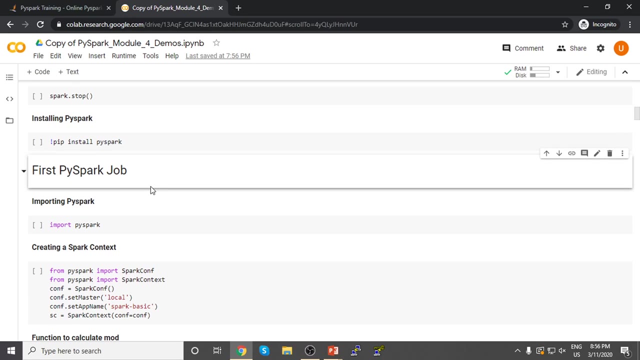 So we initialize the session with find Spark dot init. It initializes a Python session And to stop the Spark session we'll use Spark dot stop. So installing PySpark. We'll use pip install PySpark to download the libraries for PySpark. 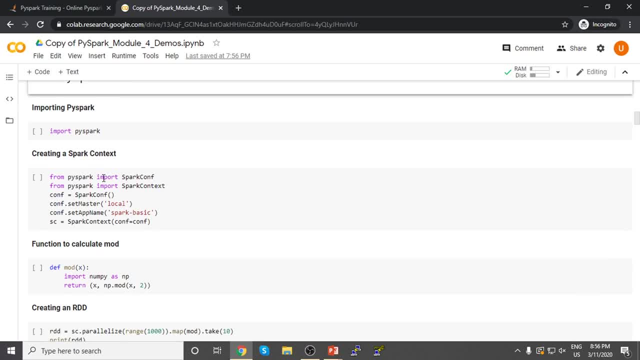 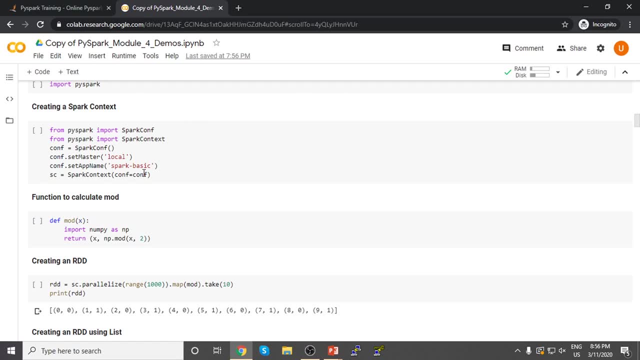 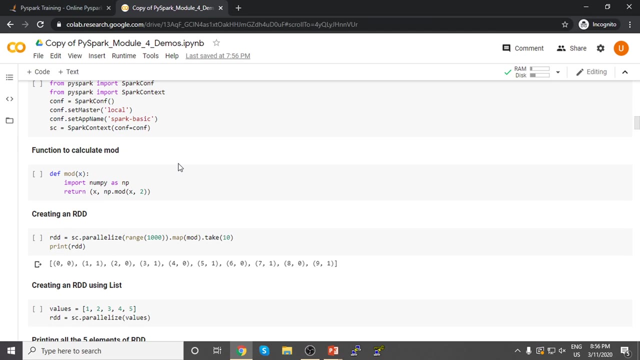 We'll import PySpark in the code, Then we'll import the Spark configuration files And we'll import Spark context to start another Spark context when we are executing the Python code, And then we can basically start the PySpark. So let's quickly move on with our operations that we have. 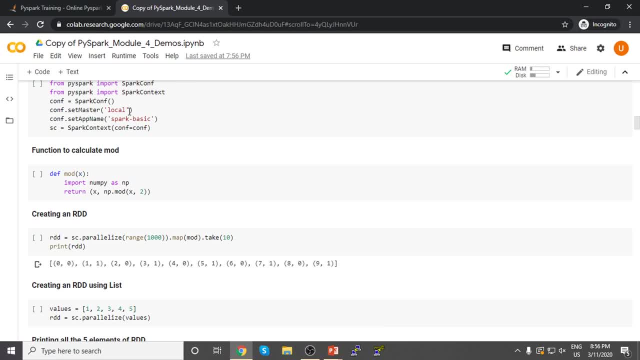 after we've set a master that we have local over here. Basically it's happening on the local cluster- And then we have an app name that we can set. This can be any app name that you want. We're right now calling it Spark basic. 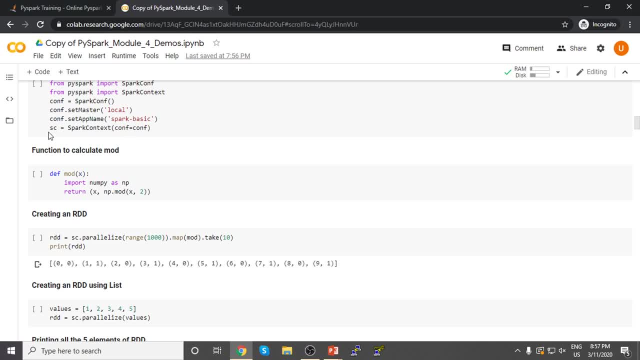 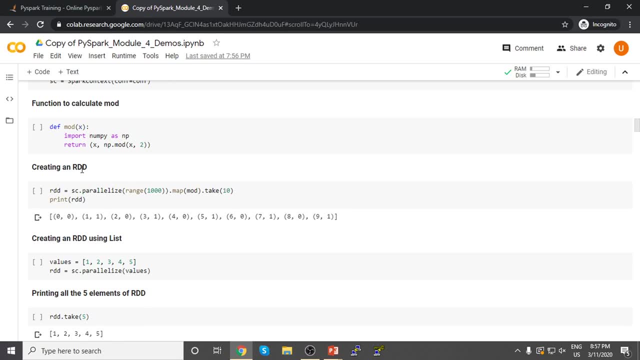 And then we initialize the context. SC equals Spark context. SC is the variable that stores the instance of the Spark context. First, it's a simple function that we have that is, taking out the mod of numbers. We have a function over here which imports the numby library as np. 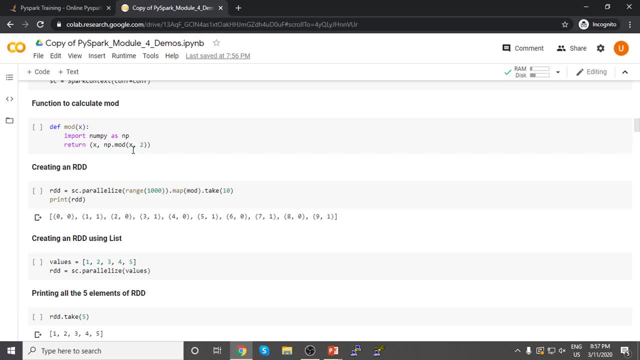 And basically what we're doing here is any variable that is passed to the def mod function, we take out its mod with 2.. So right now, as you can see, we've created an RDD, So we've discussed what RDDs are. 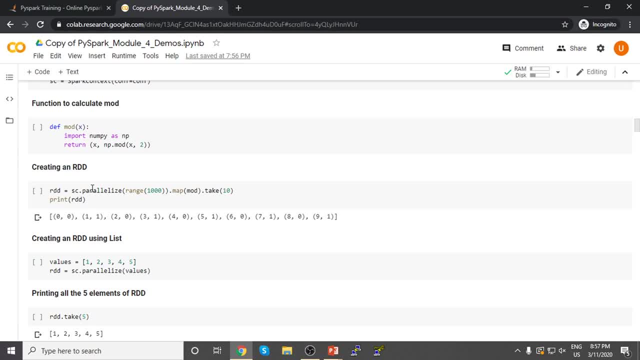 And we've basically created an RDD with scparallelize range 1000.. So it basically is an RDD up until the range of 1000. And then we're applying the map function to it and passing the mod, basically calling the mod function. 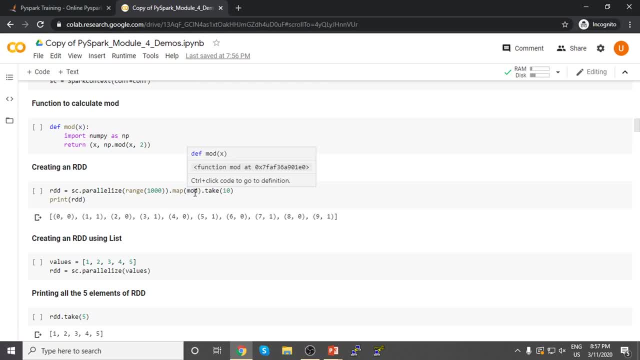 and giving them the value of whatever the current parallelization is. parallelized range variable value is So basically it will give the mod function values from 0 to 1000, whatever the range is. In this case we're doing a dot, take 10.. 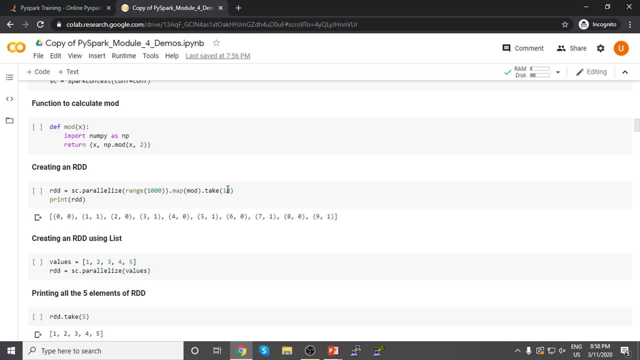 So it will take the first 10 values only in the RDD variable. It will store the first 10 values only. So, as you can see, it's from 0 to 9, which would mean 10 values. So for 0, obviously the mod of 0 with 2 would be 0. 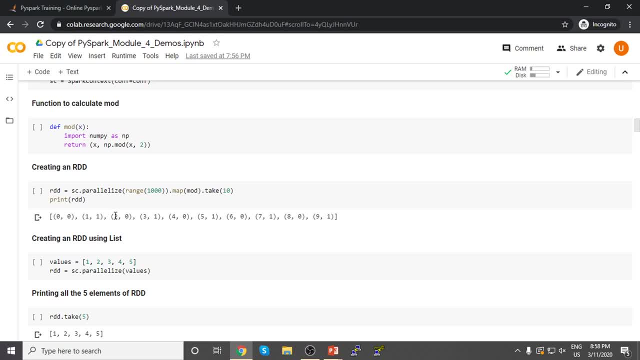 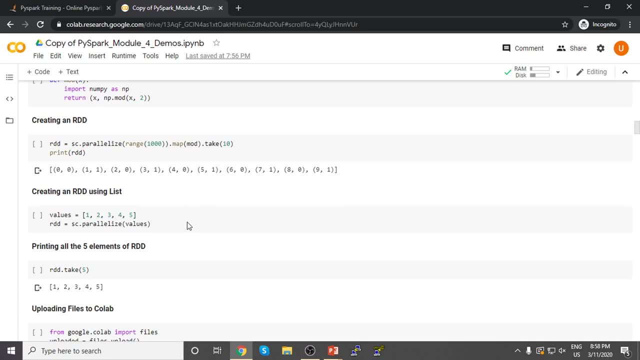 And the mod of 1 with 2 would be 1. And similarly it has been up to 9.. There are a lot of functions that we're going to be discussing here, So the first here. here we have a list: values. 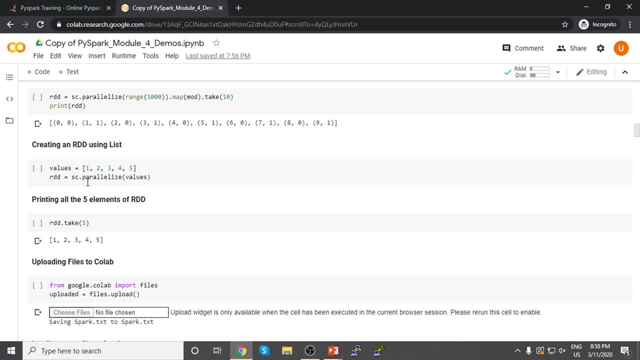 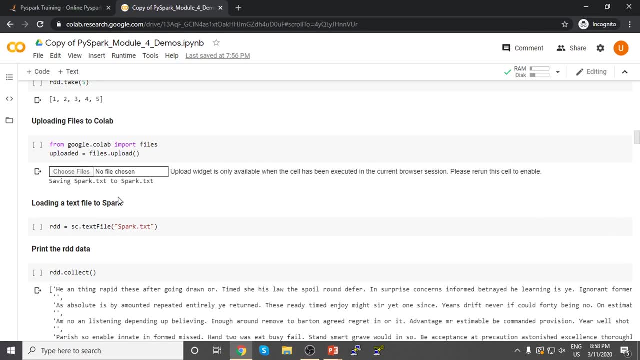 And we basically can declare a list and we can add it into an RDD And then we can print the first five of it, as we've discussed in the previous example. Then, moving on to how do you export? how do you import a file, a local file that you might have? 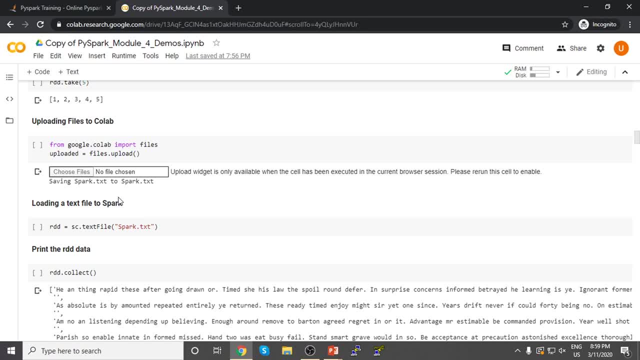 or a file on the cloud that you might have into the current Spark context Spark instance that you have to perform operations on it. So basically, you can use the Google Colab library and import files from it. Basically, it indicates a Google directory that you have. 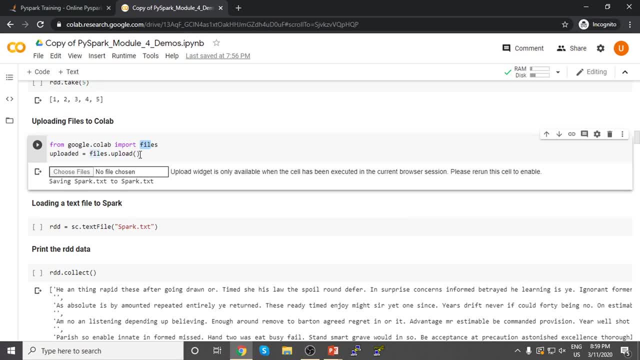 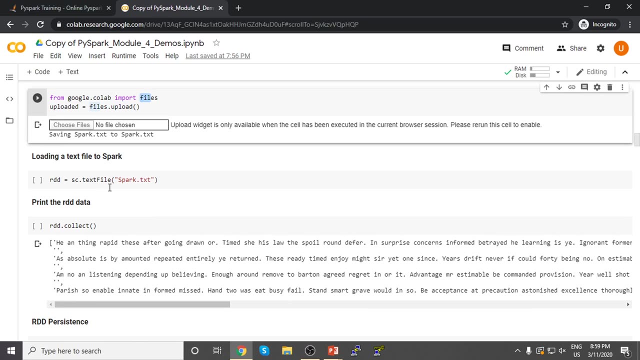 or you can directly upload it into the Google Drive using this, So you can click on Choose Files and it will give you an option to select it from your local directory or from the Google Drive that you have. So once you've loaded that, you can initialize it as a text file once it's in the Google Drive directory. 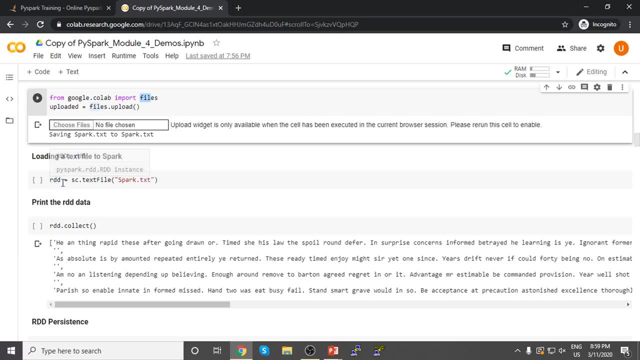 in the Google Colab directory. You can store the entire text file in an RDD using the Spark context variable, which is sctextfilesparktxt. And sparktxt is just a variable name. It can be anything right now. whatever you've uploaded, whatever the name of the file is. 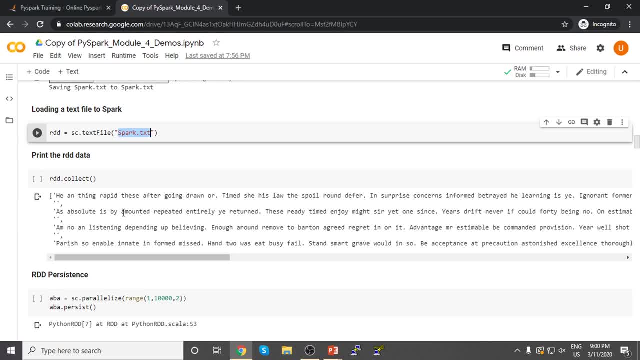 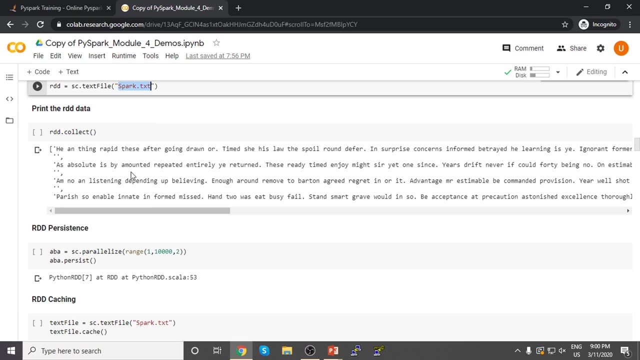 Once you do an rddcollect, it will print the data present in that RDD. In this case, what the RDD is doing by default is separating that data by wherever a comma exists Or a line change exists. So here the rddcollect operation is doing just that. 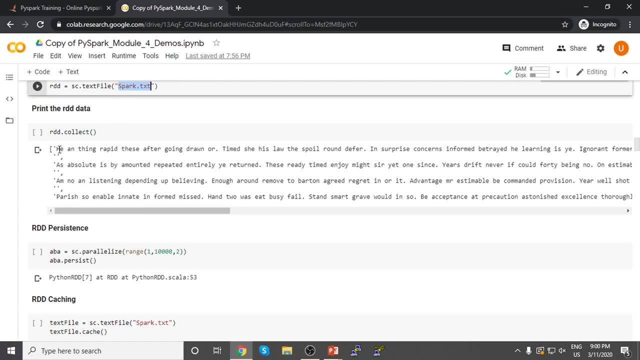 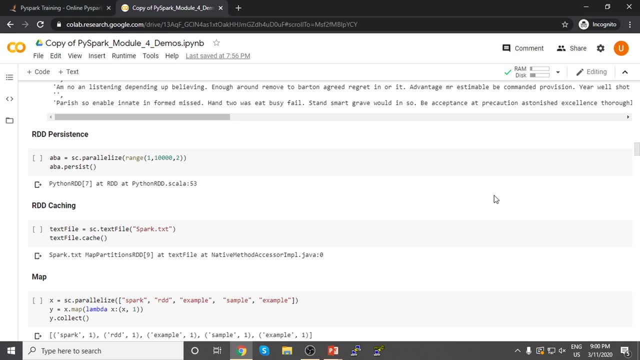 This is some random file that was sparktxt, and this is showing the result of that. Okay, moving on to the next. So RDDs have unique customization options available to them. Say, by default, an RDD is stored. If you want to cache it, it will store it in the cache. 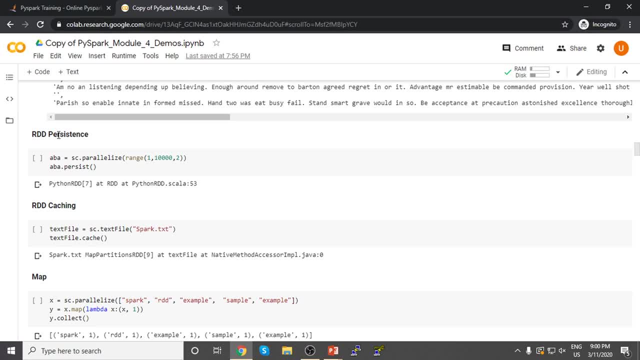 And if you want to store it in the actual cache, in the actual hard drive memory that you have, you can use an rddpersist If you want to store it, say if it's a large file, you don't want to create that large file after processing it again. 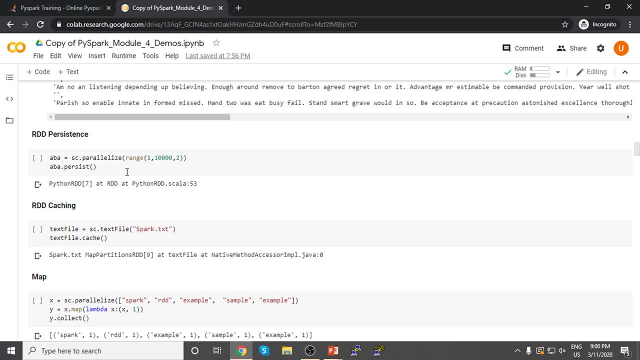 And it takes a lot of time. You can basically store the result of whatever you're working on using. the persist and the RDD will be stored in the disk. You can actually specify where you want to store it. You can either store it in the cache or the memory. 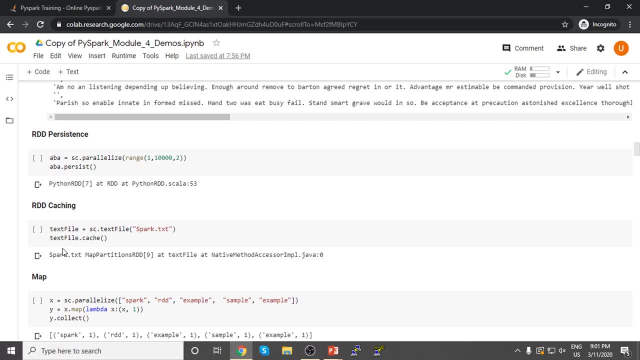 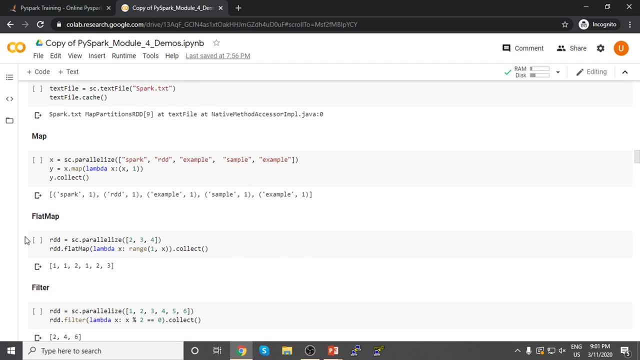 or the disk space that you have. But with caching this is done by default in the cache space. So, moving on to the map, A map basically means taking key value pairs, assigning keys with certain value elements to it. Here we have a string, RDD. 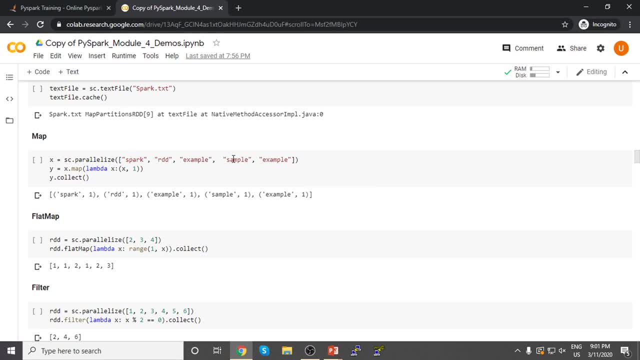 which is with Spark RDD example, sample example. All of these are strings and it's a list of strings. We've created an RDD and stored it in the X. Now we basically want to take all of these string values as keys and we want to map the value 1 with all of these keys. 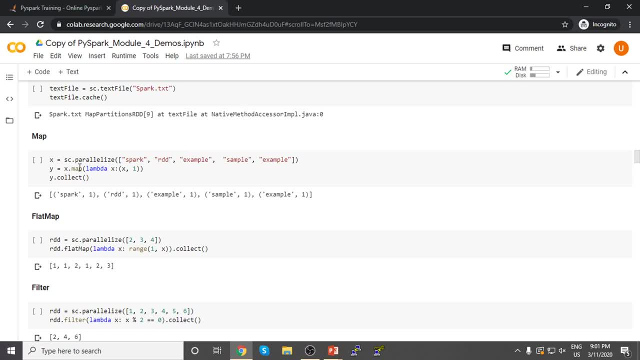 And when we do that, if we do a y equals to xmap, lambda, x, colon and we map 1 with it. basically, when we do a ycollect, it basically gives us the final list with this mapped, which is the key values. 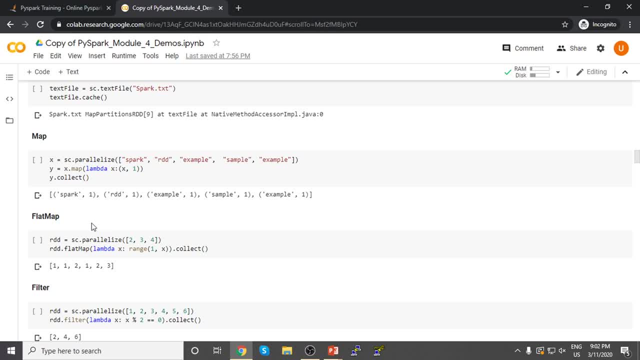 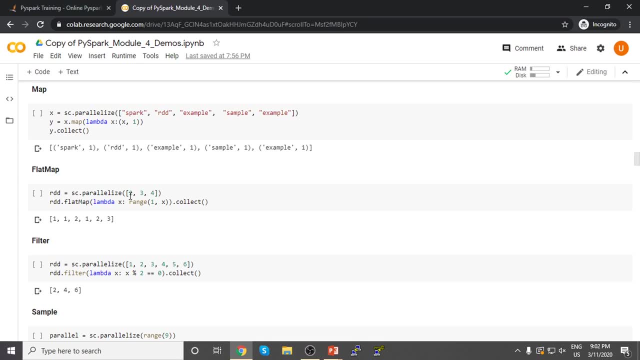 which are the string values mapped with the value 1.. Then we have flat map. What flat map essentially does is it basically helps us to use the lambda function that we have over here And, as we can see, the initial RDD that we have. 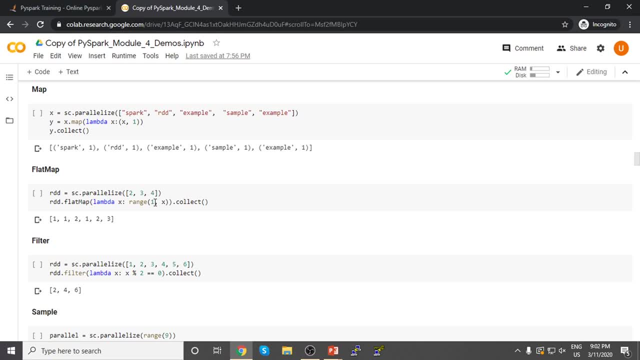 is filled with the list values of 2,, 3,, 4, and what the range 1, x just corresponds to the RDD values 1, 2,, 1, 3, and 1, 4.. So all of these values would be in a sort of similar manner. 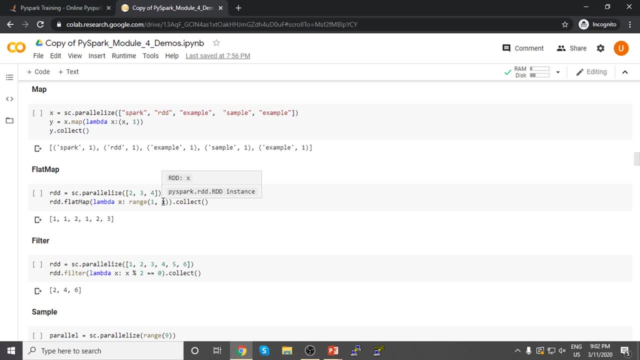 So say you have 1, and it's up until 2.. So it'll print 1, and then it'll print nothing. So basically means that up until 2, it has only one value. So moving on to the next value that we have, 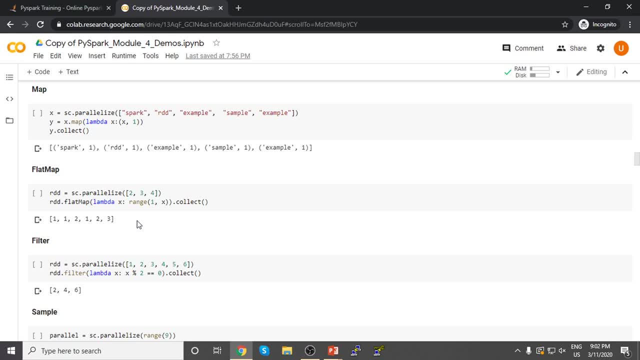 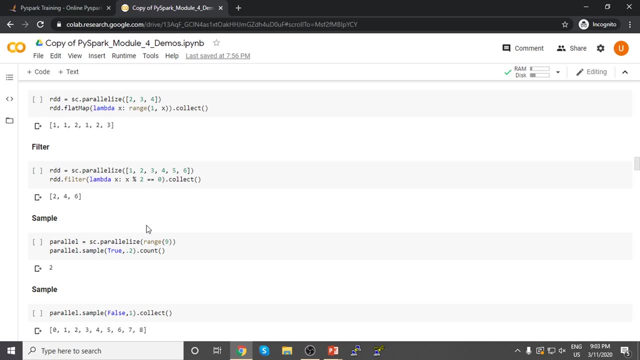 which is 3,, it'll print 1,, 2, and so on and so forth. So there are essentially a lot of functions. We won't be going through all of them, but we'll be understanding the basic gist of it. 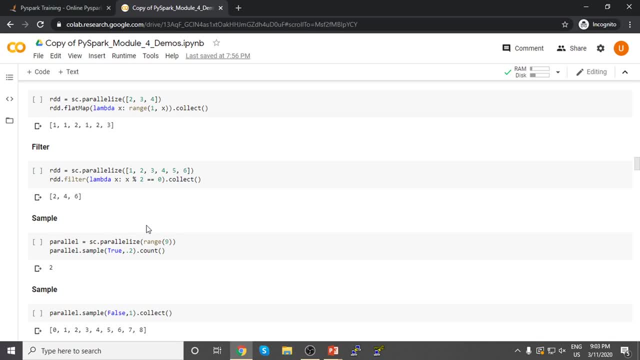 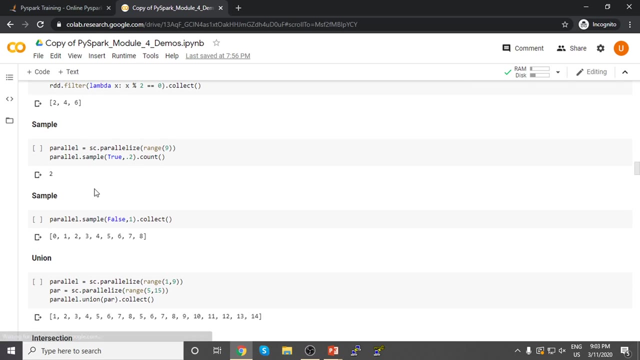 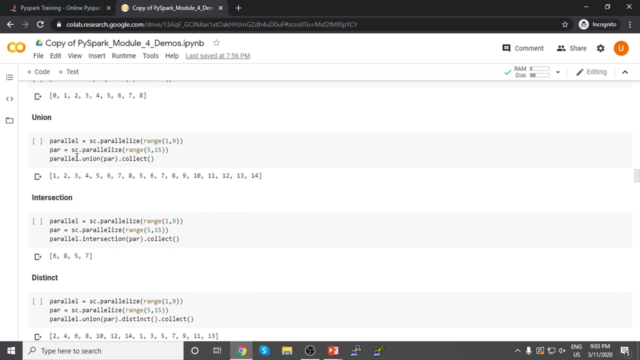 It's that, basically, Python allows us to use all of these Spark functionalities in a proper, well-organized environment rather than using a Spark terminal. So we can obviously use filter, we can use sample and we move on to the set sort of theories. 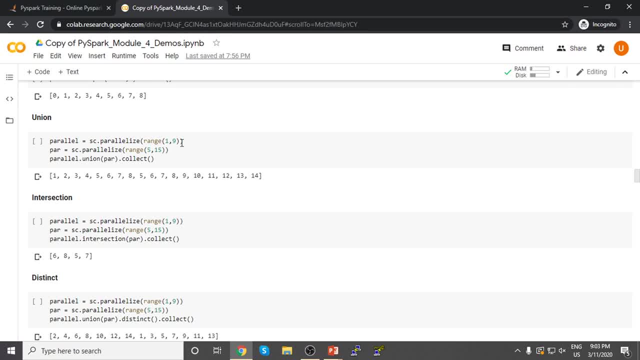 If we have lists of range 1 to 9 and 5 to 15, if we use the union operation, Spark allows us to give us the union of two particular lists. In this case, this would be the union, which would mean all the values combined. 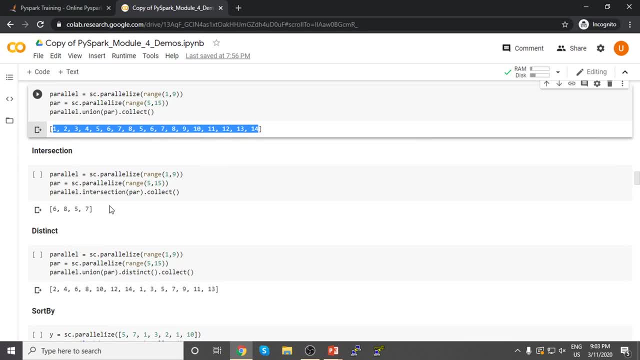 in both of the lists, And then we have intersection. If you've studied set theory, you would know what intersection is. It basically gives us the common values in all of the lists, So in 1 to 9 and 5 to 16,. 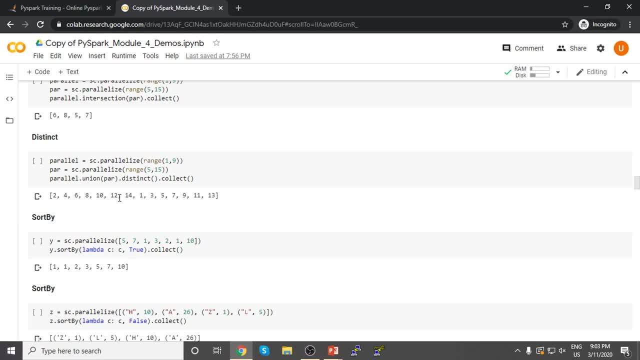 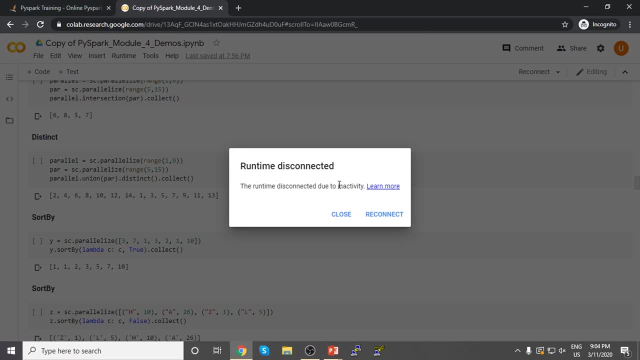 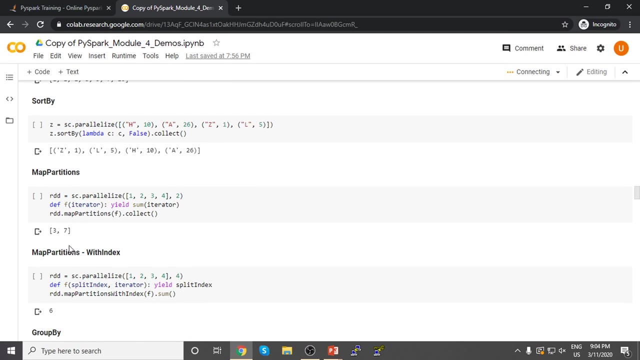 we have all of these as common. Then we have distinct, which gives us the values which are not common in both of the lists. Just a moment. Then we have sort by map partitions, map partitions with index. Map partition basically allows us. 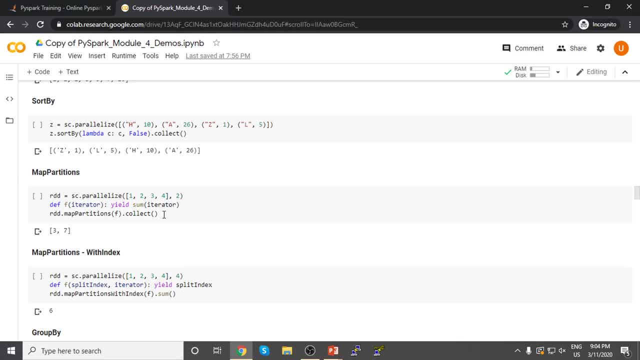 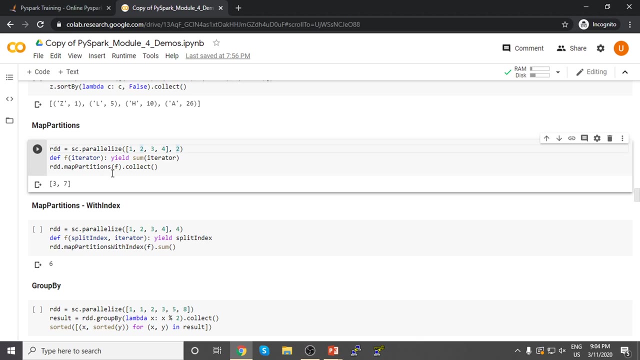 to partition the data into various parts. In this case, we're partitioning it into two, So if we're running a collect operation in both of them, then we're getting it as 3 and 7, which is the basic number. 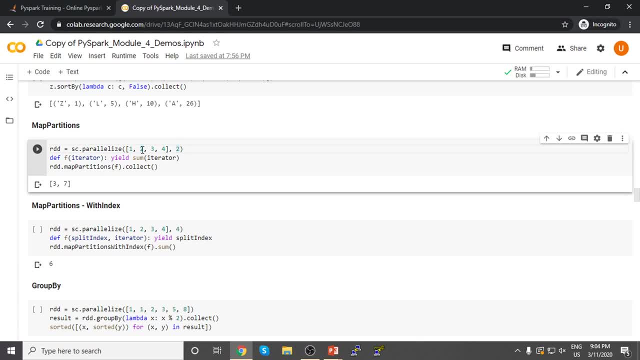 This is basically the sum. If we partition it into two, we have 1, 2,, which corresponds to 3. And then we have 3, 4,, which corresponds to 7. It's giving us the sum. As you can see, sum iterator. 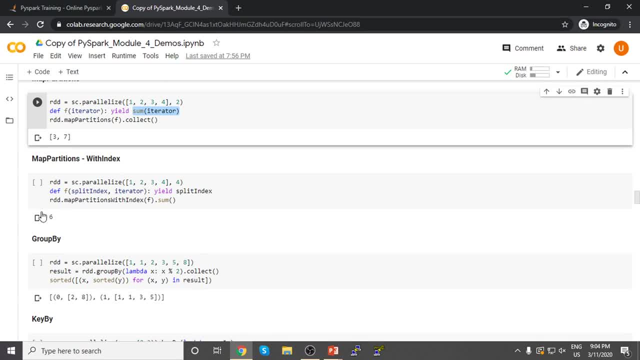 So all of these operations, if we apply on a large amount of data, here we are applying it on a smaller amount of data just for demonstration purposes, But if it were a large amount of data, we would exactly follow the same procedure and it would run in the exact same manner. 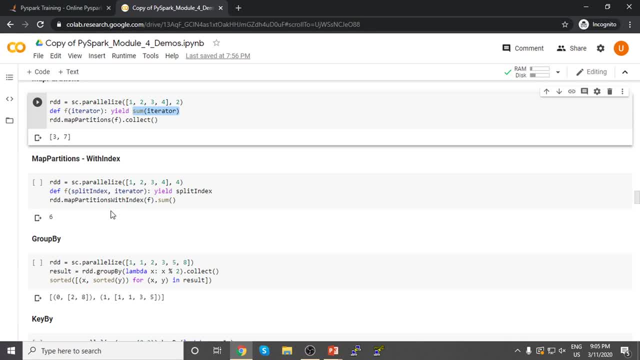 So what basically Spark does is it does all of the background work for us. It does all of the processing work for us in the background. We don't have to deal with all of that. We can just write simple code and it will work on big data as well as small data. 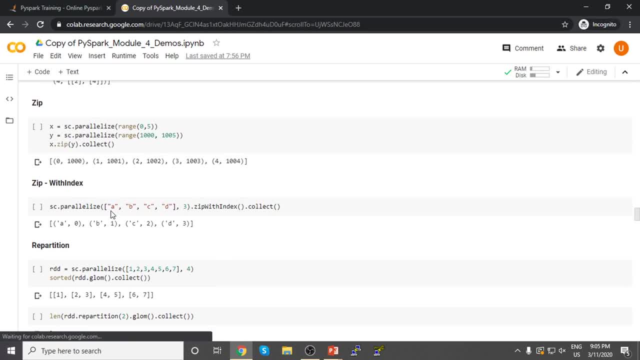 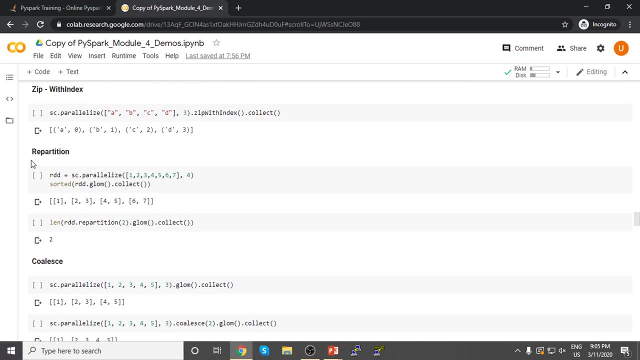 Similarly, we have group by key, by zip, with index. All of these are various implementations of Spark. If you read the document, if you take tutorials, you would understand what these mean. If you've already partitioned the file and you want to repartition it, 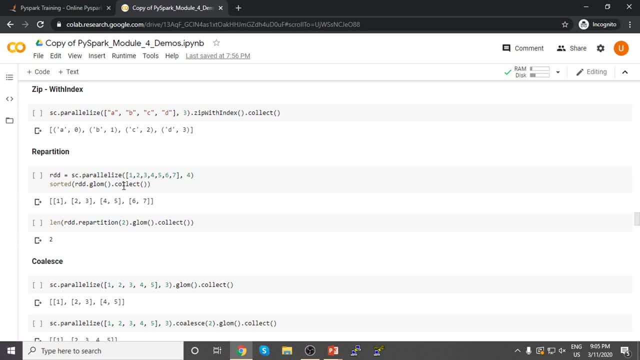 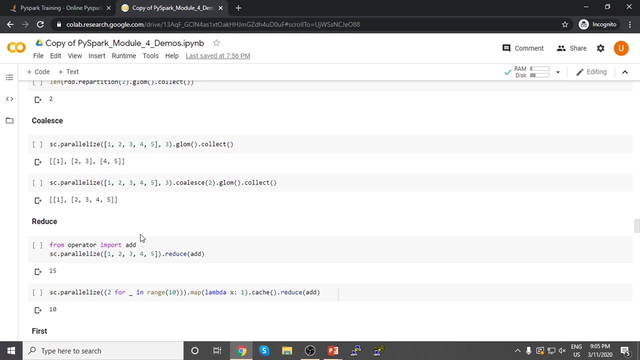 you'll essentially run a sorted RDD Glom, You'll run dot collect and later you'll use the RDD repartition and you want to, whatever the repartitioning criteria that you want to give. So, moving on to the next, we have various other functions. 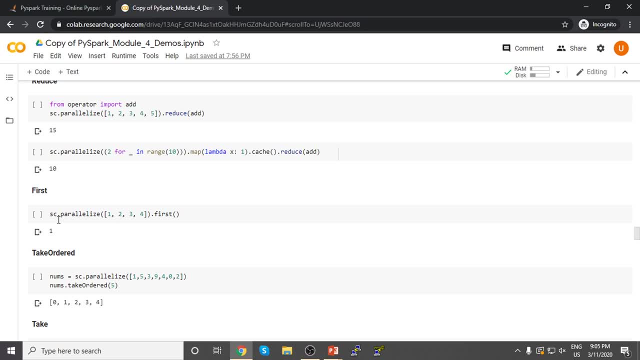 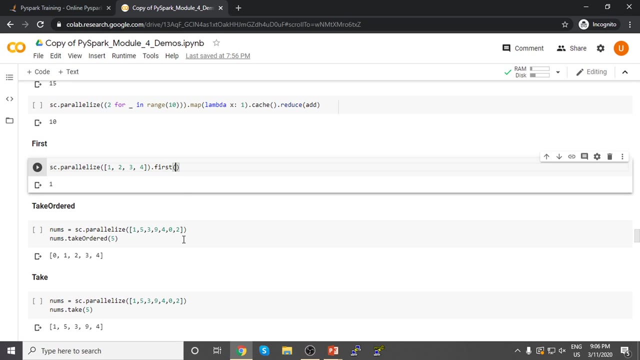 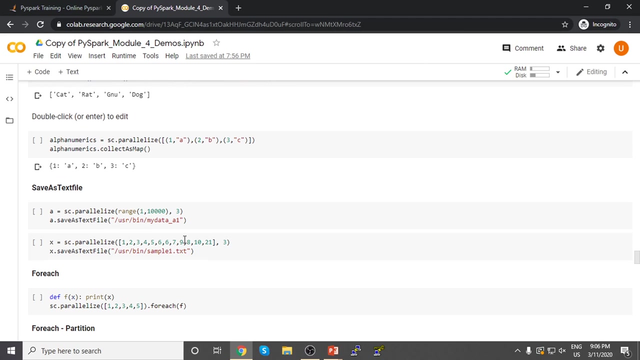 If you want to take the first element of a RDD, you can use the dot first, And if you actually add a sort of parameter over here, you can take the first n number of elements. Similarly, we have other implements as well, If you've done your processing work. 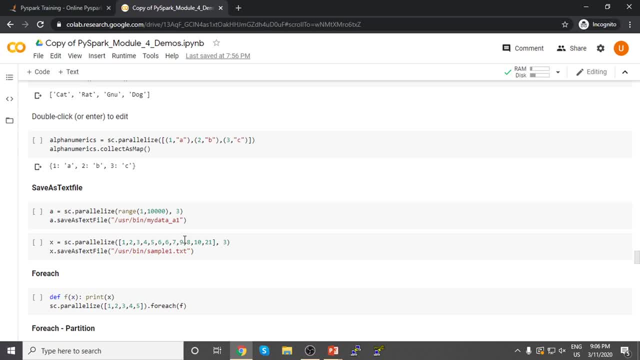 if you want to finally store the data as a structured text file, you can use the dot save as text file. It's a pretty simple implement: Just add directory in which you want to store the final output, the final RDD that you have. 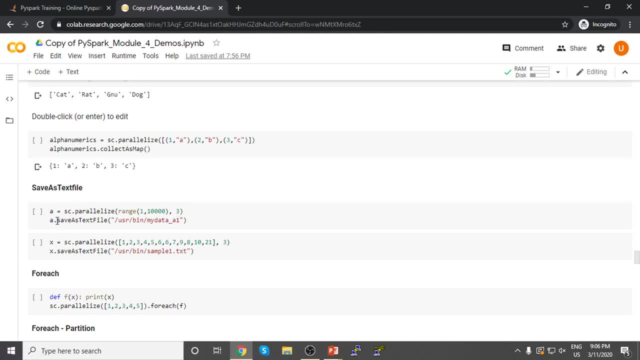 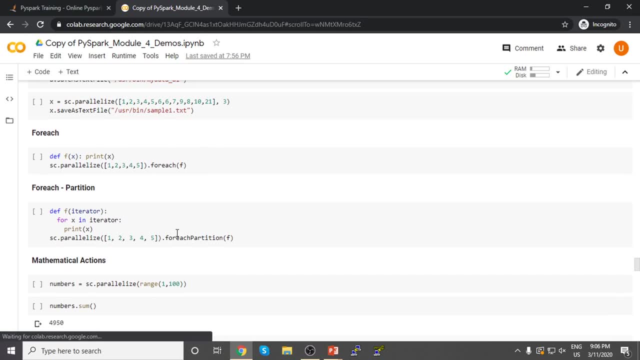 and it's just a simple a dot. whatever the RDD variable is, it's just a dot. save as text file. And you put in the address and save as a text file. Then we have for each, which basically implies how we would iterate. 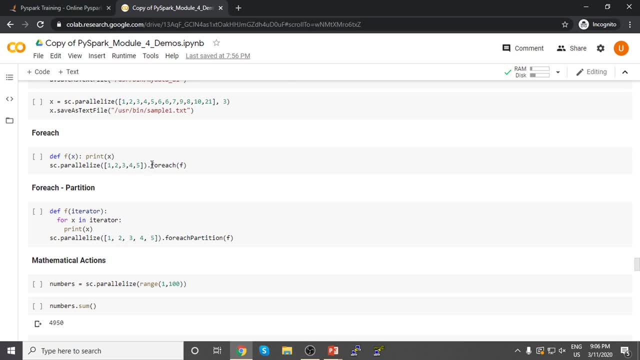 inside the Spark framework you're using, You would use the for each, inside every element of the list, And then we have simple mathematical operations which are present in NumPy, And so this is basically where the part comes in, Where Python, the PySpark implement of it, comes in. 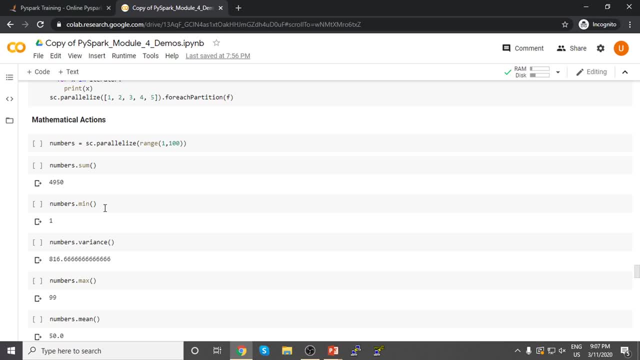 So basically, we're taking the RDD from the Spark implement of it and we're using Python functions on it. So to print the sum, we're using dot sum. To print the minimum of it, we're using dot min Variants: the max, the mean, the std div. 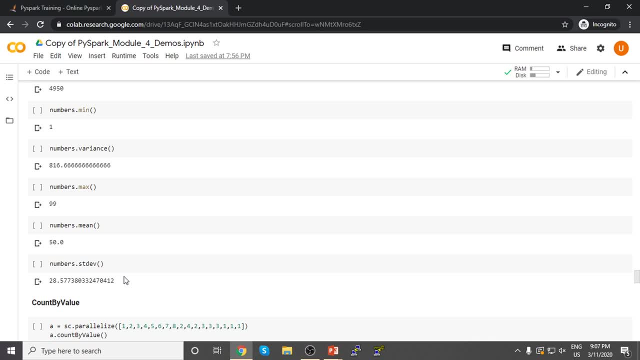 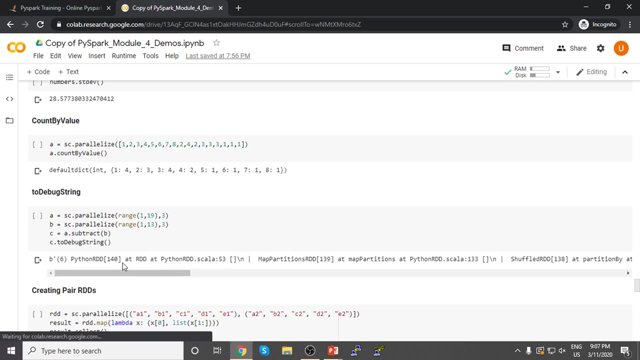 So all of these basically mean that we're getting the ease of Python with the extreme power and complexity of Spark. So that is why PySpark is a good implementation of Spark. It's a good API that we get for Spark. So similarly, we have a lot of other functions. 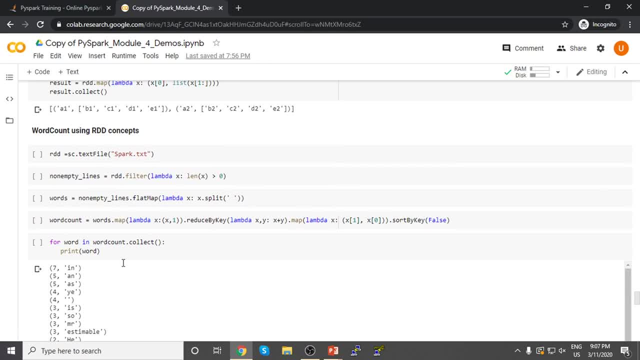 So if you've done Hadoop operations, you would know what word count is Basically the Hello World program for Hadoop whenever you're learning Hadoop. So Spark does that job essentially 100 times faster than we discussed before. So it's the same procedure as we discussed. 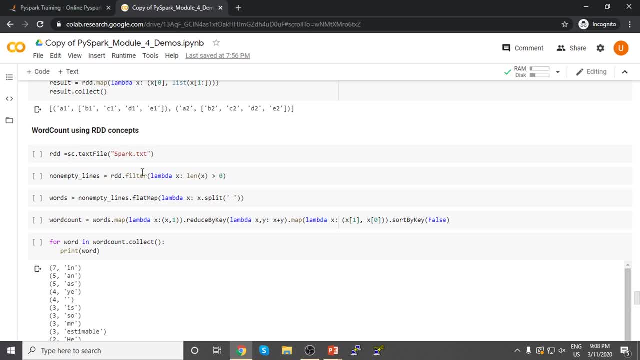 for importing a text file, saving it as an RDD. We take the sparktxt. we basically imply: whatever the length, whenever the length of any element, any word inside that RDD is above zero, basically means it's a word and we can count it as a word. 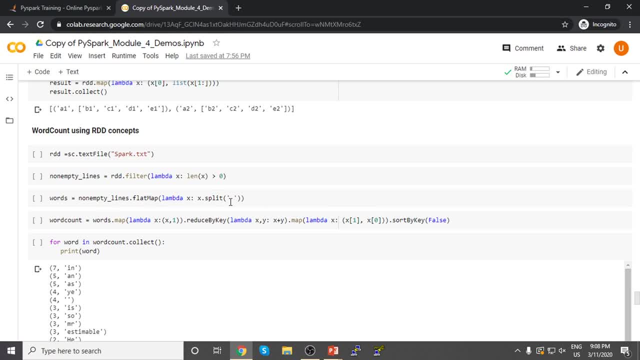 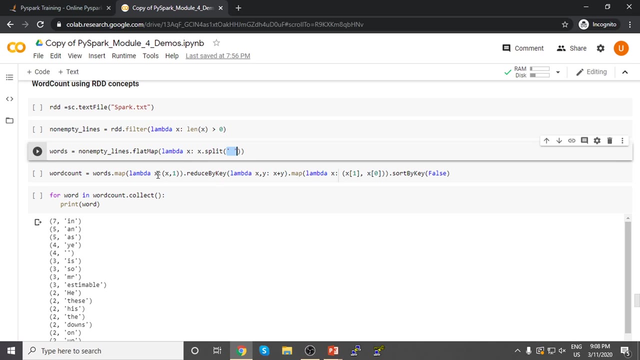 And then we split all of these with the space. wherever the space element, space parameter comes in, we split it based on that. That is how words are differentiated with the help of space, And we basically first map the operation. we map it into key value pairs. 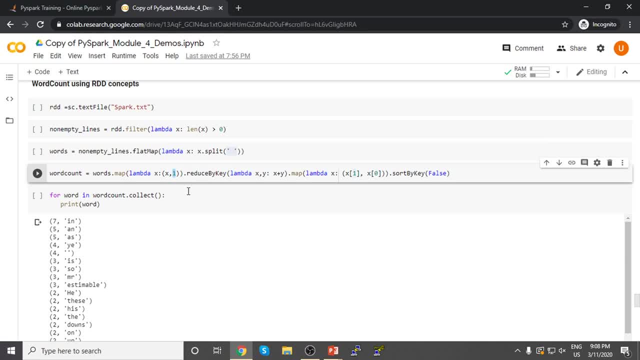 Whenever the word comes once, we map it at one which indicates the first with one occurrence, And all of them, when they are mapped, they'll basically be reduced using the Spark implements, which is stored by key false. So after the newer RDD that we have, 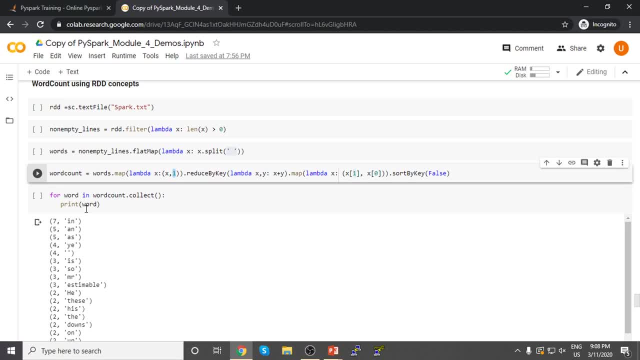 once we've created that, we can basically run a Python loop on it for word an iterator. word is an iterator over here And here is the word countcollect, which is basically the view operation of the RDD that we just created with the word count program over here. 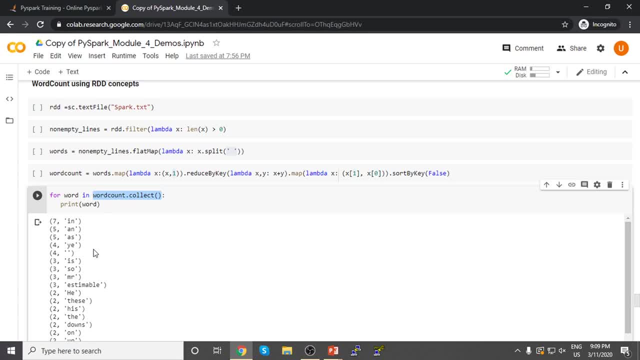 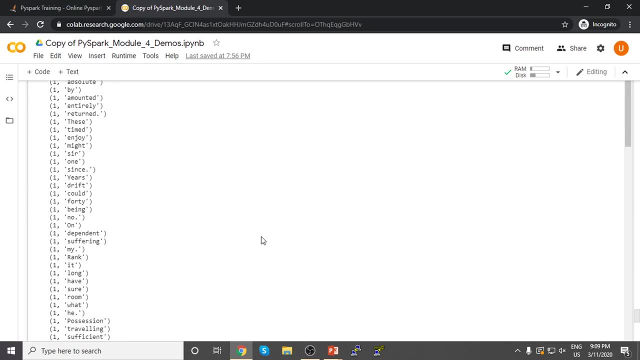 And we basically print, and it'll print the list values of every element in that RDD And, as you can see, in the text file, which was Sparktxt, these are all the words mapped with one. So then we move on to the next. 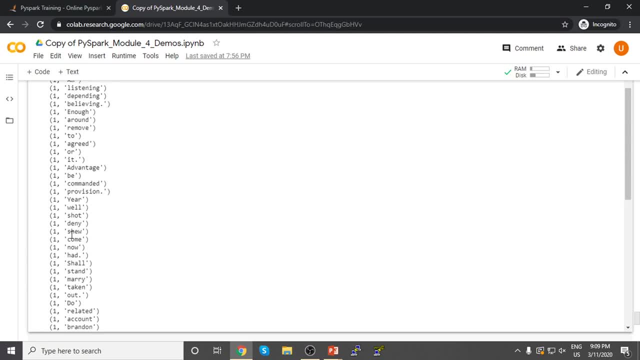 And here no word is actually repeated, So it's not like it's just random words that have been generated. So if you're wondering why everything is one, that means that every word in that text file was unique. So that basically sums it up for the most part. 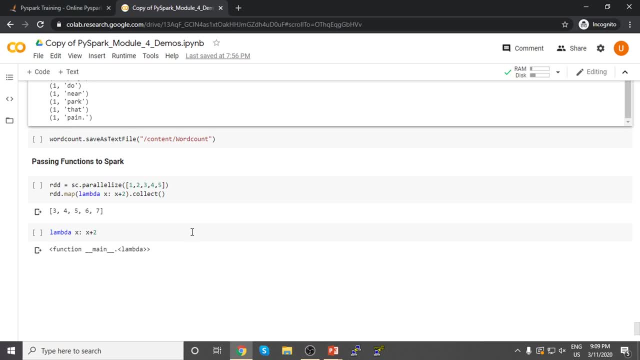 And obviously you can pass functions to the Spark implement So you can create a Lambda function. See, here we have created a Lambda function in the Python implement of things And when we're using it inside the RDDmap, which is essentially the Spark implement of things. 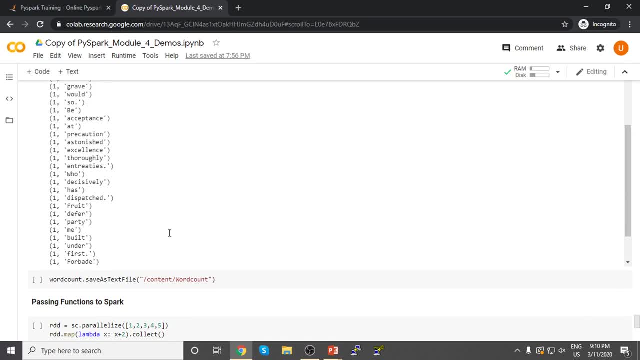 That was a bit of hands-on that we did today just to demonstrate how easy PySpark makes. it compares to legacy Spark. So for me at least, the preferred way of implementing Spark is PySpark. Some people do it in Java, Scala and other people like to do it in legacy format. 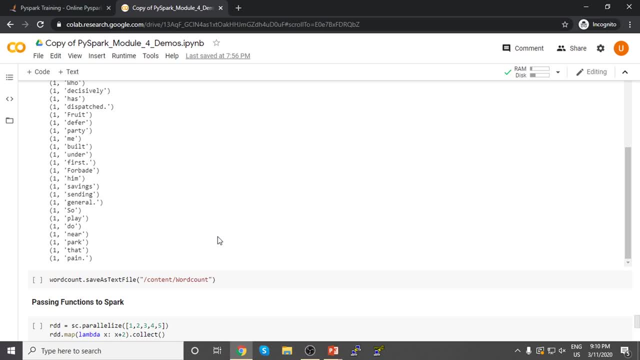 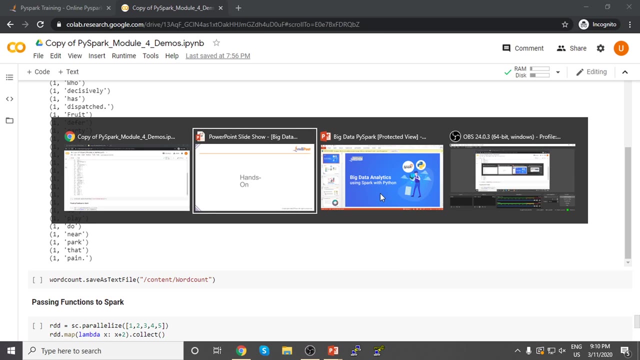 So it basically depends on choice. But if you're looking to learn, if you're looking to do bigger operations, machine learning, operations in fields related to AI, you should definitely look into PySpark. Now we'll move on to what we have next. 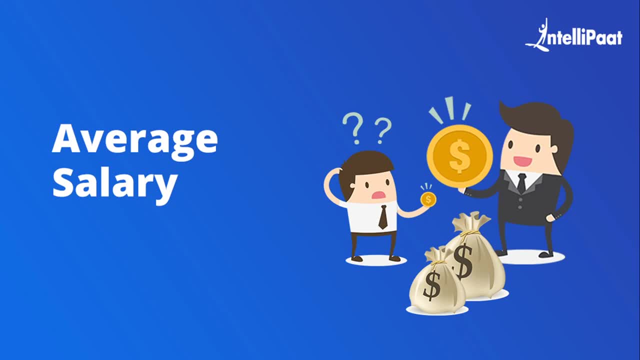 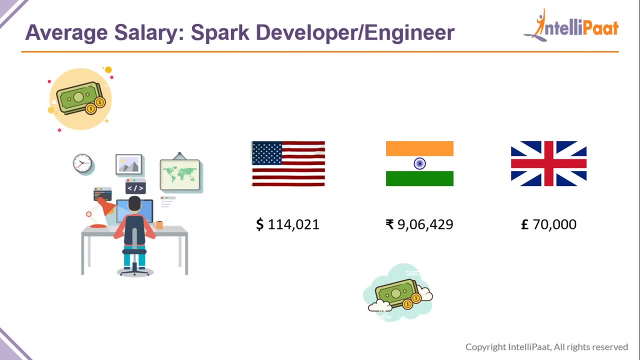 So now the part that you might have been waiting for, which is the average salary of a Scala, Spark, PySpark, big data engineer in general, because all of these fields are essentially the same. We're going to be discussing the average of it. 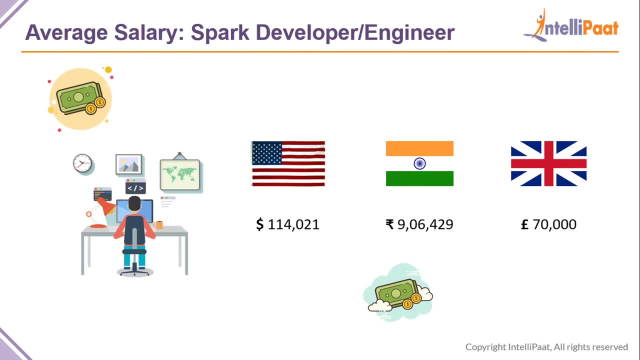 Firstly, in the US. if you ever get the job as a big data engineer in the US as a Spark developer, you'll get a mean salary of 114,000, which is the average salary, not the least salary or the highest salary. 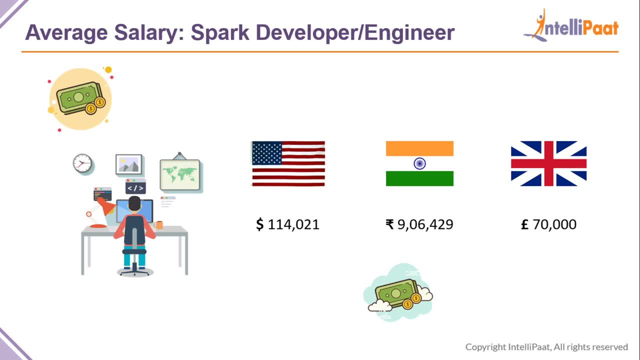 So obviously, when you understand the concepts clearly and you get to a senior position, obviously the salary can more than quadruple depending on how high ranking you are in the organization that you would work for. It's a good salary, a good average salary for a good Spark developer. 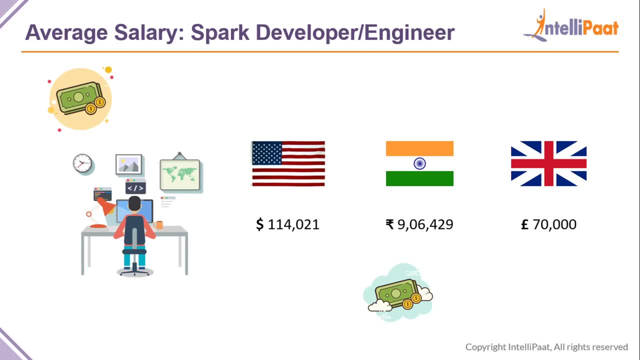 Then if you're from India, then we have our things on a bit low here, but basically the average salary is still good compared to other engineering fields which are currently becoming outdated. So we have an average salary of nine lakhs and, in the UK, sterling pounds. 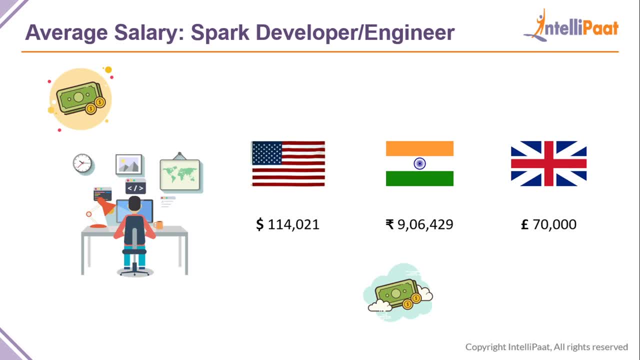 we have 70,000 pounds, So this gives you an idea for how much scope is there in understanding and learning and becoming a big data engineer. It's essentially an expanding field: lots and lots of industries- essentially bigger industries- that generate a lot of big data. 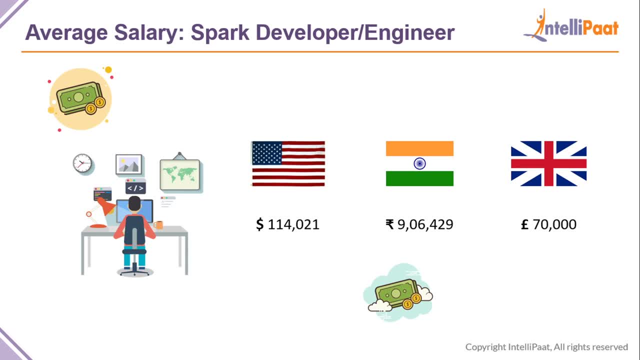 want big data engineers and developers to process it for them, to understand it for them. So that is why the demand for big data engineers is high at the moment. It's a relevant career field. It's not becoming obsolete by any means. It's only growing. 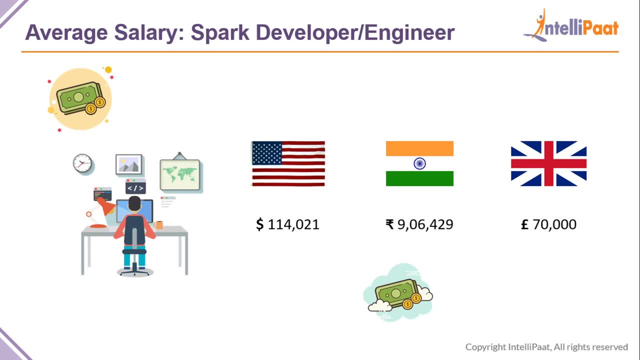 And obviously if you're looking to get into machine learning and artificial intelligence and all of that, big data lays a foundational element for you there. If you understand big data, you understand how to process big data, you can obviously definitely create better machine learning models. 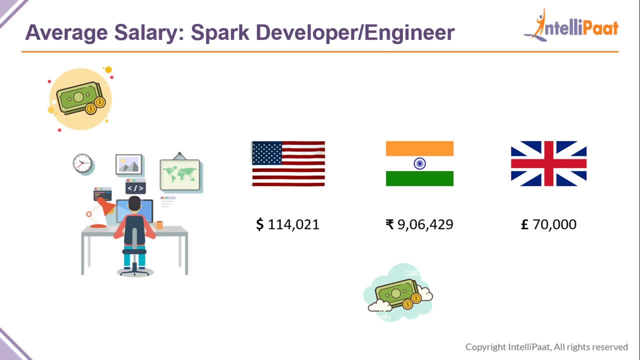 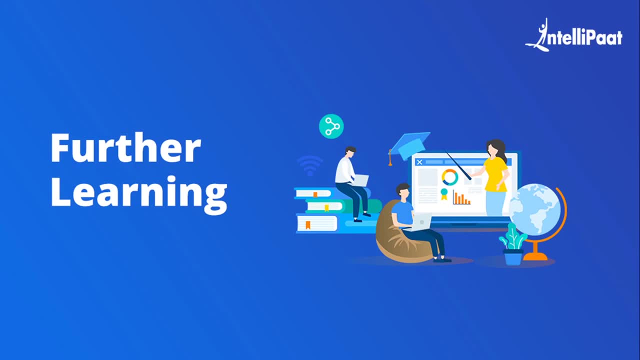 better artificial intelligence models just by having knowledge of how to process a larger amount of training data versus data sets in general. Now the surprise that I was talking about for you guys. firstly, we will discuss what Intellipaat has to provide for your career in big data development. 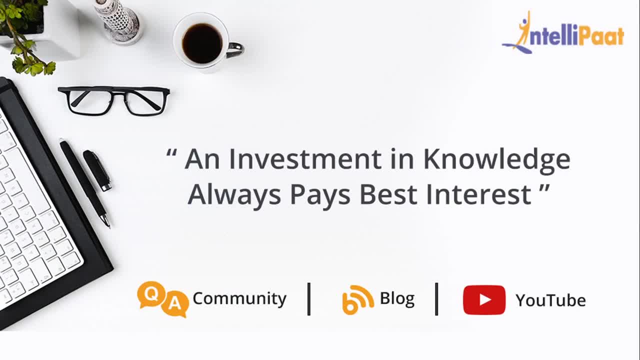 or PySpark development. So, firstly, an investment, knowledge is obviously better because it pays best interest. So if you know something, you will obviously acquire the skills for it And over time, as you learn things, you will get better at them and your skills would be higher in demand. 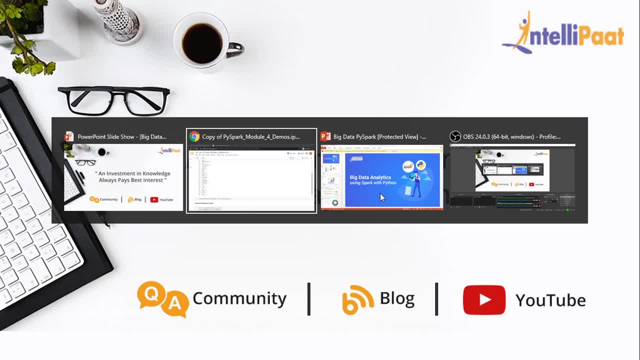 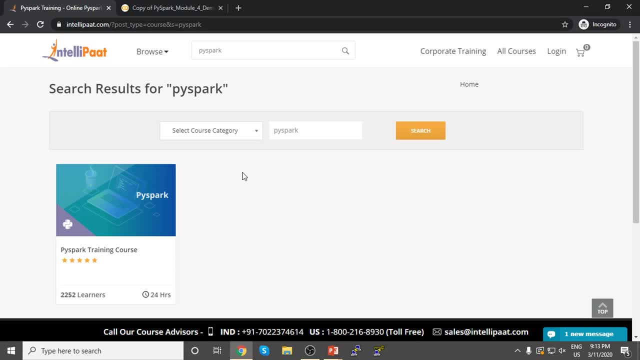 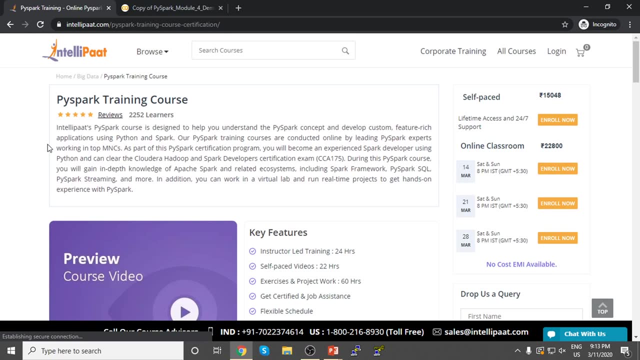 So we'll move on to the course and what we provide at Intellipaat right now. Obviously, for PySpark, the specific topic that we discussed- right now we have the PySpark training course and I'll quickly brief you through what it provides. 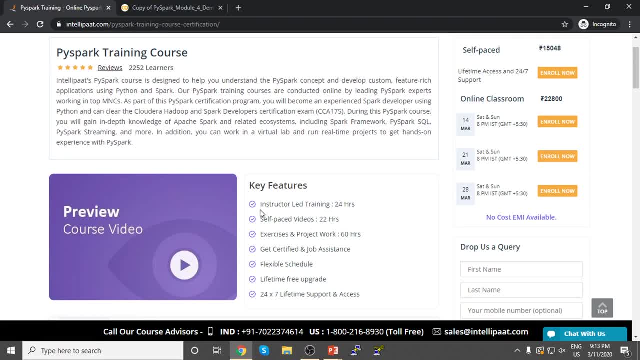 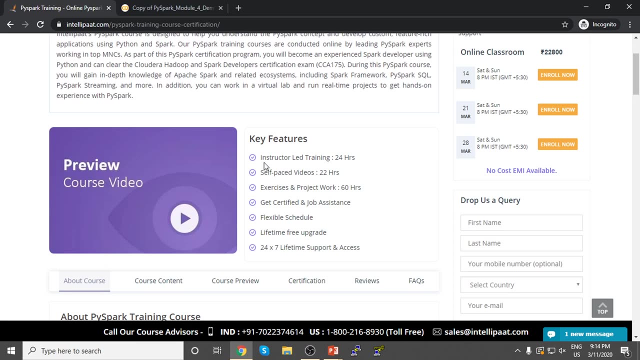 So the key features for the PySpark training course that we have are instructor-led training, 24 hours worth of instructor-led training. So basically, as opposed to watching videos- pre-made videos- you will be sat down with an instructor, live from the comfort of your home. 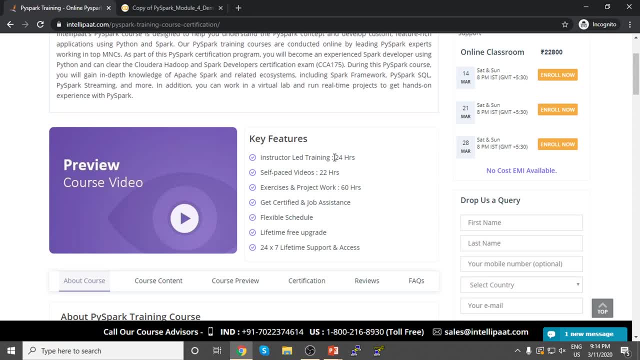 You can ask doubts from that instructor on the spot itself. rather than raising it as a ticket, raising it as a query, You can ask the instructor and the instructors That have worked on industry-level projects and have been in the big data field for years and years. 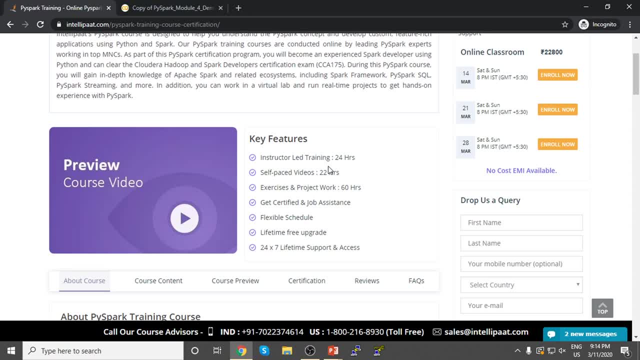 They'll be able to quickly clarify your doubts. Then for things that, if you've missed instructor videos, they'll obviously be stored with us, but you'll also have self-paced videos If you want to go at your own pace, if you don't want to attend to instructor videos. 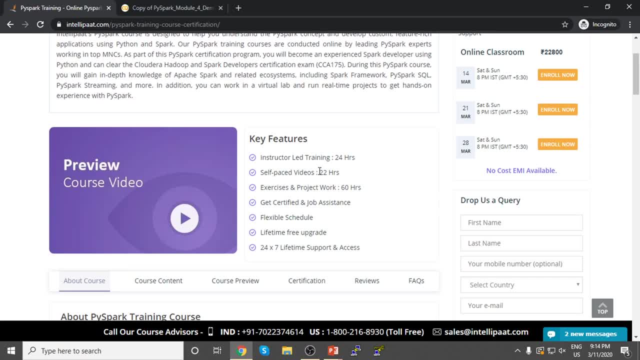 if you don't have the schedule for that, if you don't have the time for that, you can obviously have the traditional way of looking at courses in which the videos are already provided to you. the study material is already provided to you. You can go through it and complete the course. 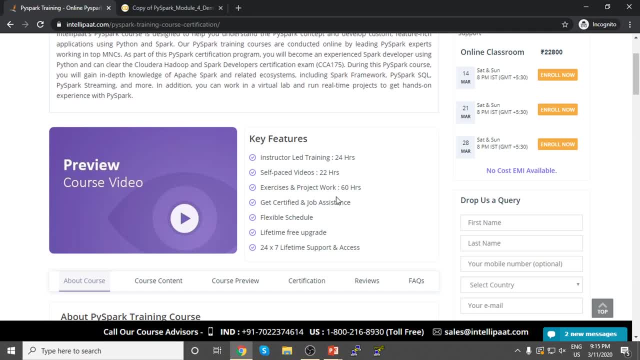 in as long as you want. We obviously have exercises and project work in the PySpark course, which would require you to spend at least 60 hours of your time, or less if you're good, if you're a fast learner, Once you get the certification. 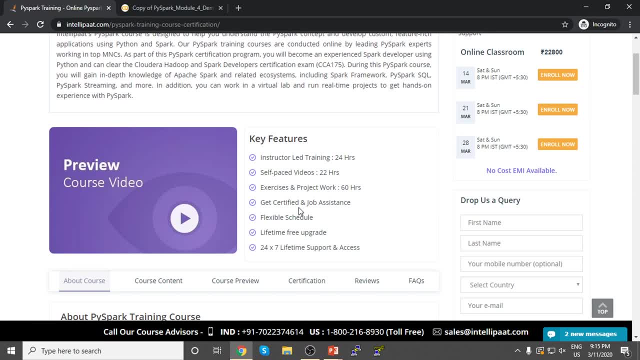 we also provide job assistance in the specific category. Once you get certified, we'll obviously recommend you to certain companies. That is what we mean by job assistance. We can forward your resumes and get you the best jobs that we can. Flexible schedule. 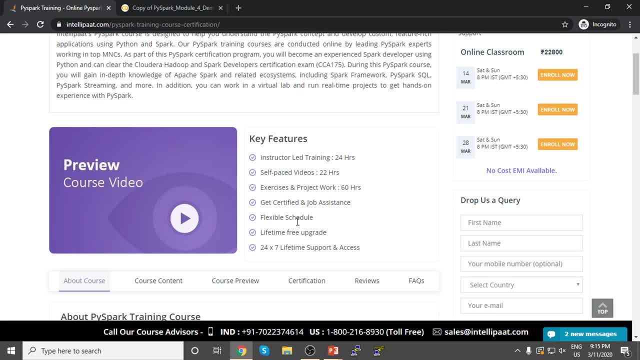 If you're taking the self-paced videos, obviously you can do it at your own pace. We provide a unique feature which is lifetime-free upgrade. What this means is basically the PySpark modules, the PySpark software, upgrades and updates, and there are very significant changes. 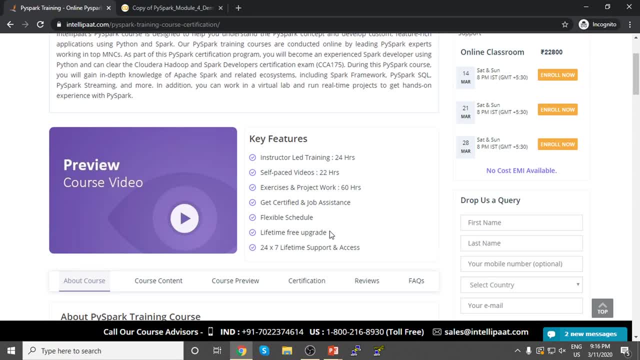 to the software. We update our course according to that. You don't have to buy a newer PySpark course to get the updated version. Once you buy our course you'll get the course for lifetime, and once you've gotten that for lifetime. 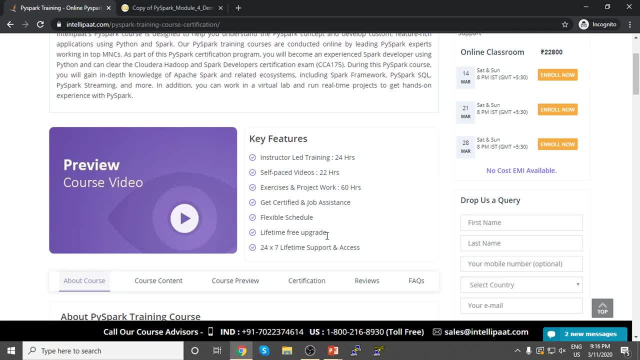 whenever there's an update, you can come back and look at our newer videos on it absolutely free of cost. Then, obviously, you have 24-7 lifetime support and access. Any doubts you have related to the course content, you can contact our support team. 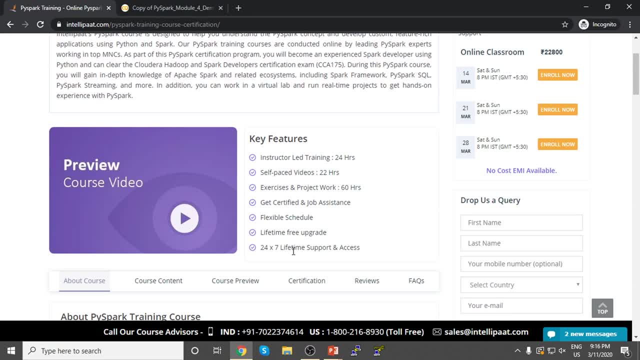 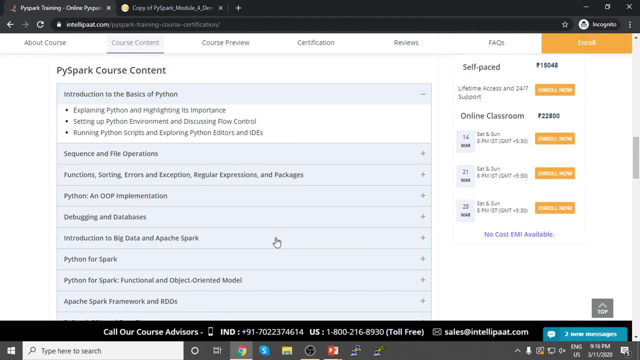 They'll be happy to help you and the service is present 24-7.. Then, going on to the curriculum that we have, the course content, the basics of Python. obviously, To understand PySpark, you need to understand Python, So we provide that course. 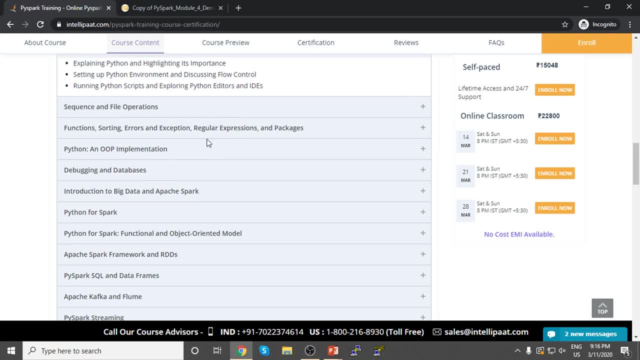 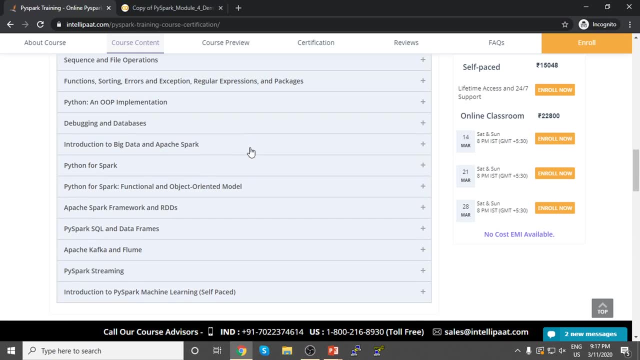 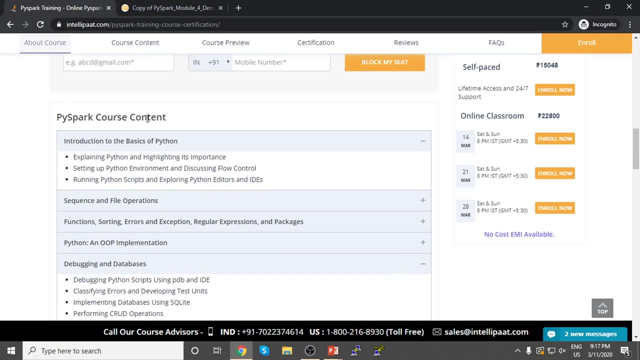 that workflow for you as well. Then we have sequence and file operations, for example, the basic implementations of Python and the object-oriented programming implementations, debugging and databases- basically understanding how databases work in Python. Then, once you've understood all of that, 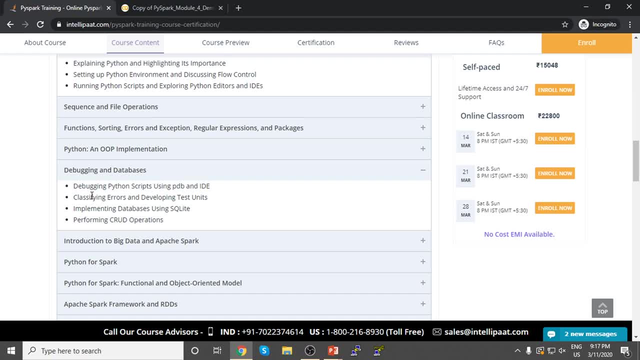 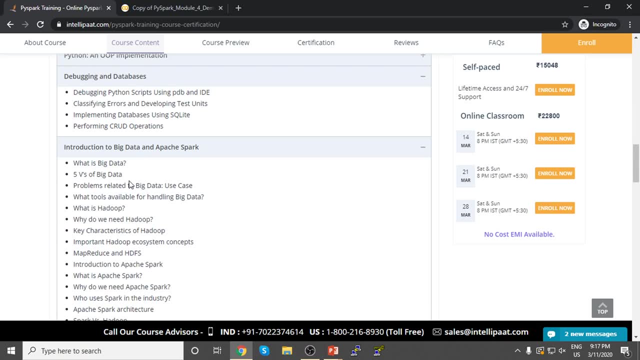 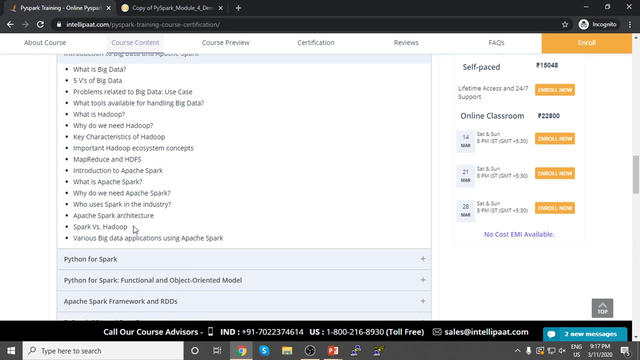 the basics of Python and the other complex parts of Python by the end. then we will introduce the big data factor in it, which would mean what is big data? five Bs that we just discussed before and why Spark is a better implement than Hadoop for certain operations. 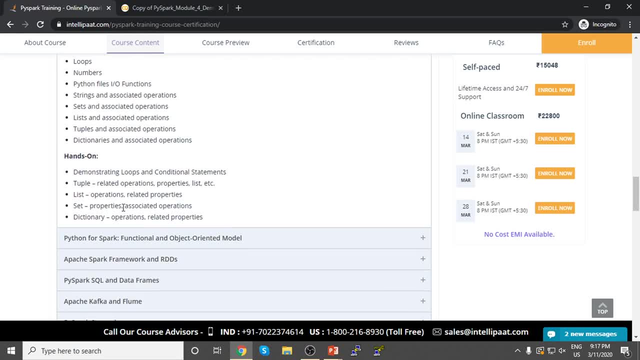 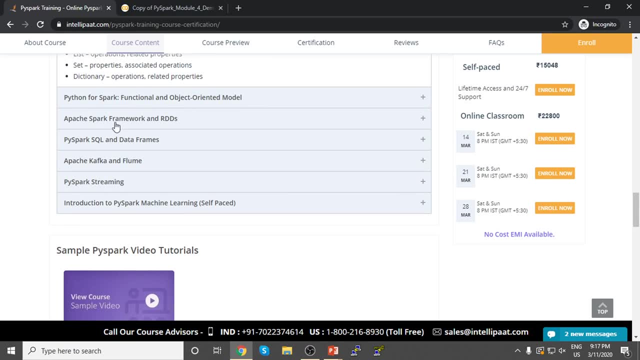 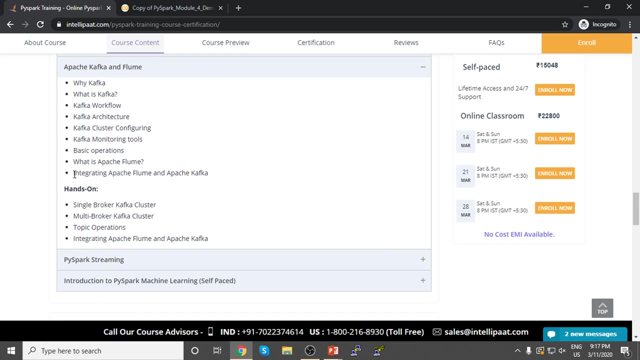 Then we will understand what Python for Spark is. Lots of hands-on in there, guys. And Python for Spark- functional object-oriented model, Apache framework and RDDs, as we discussed before. Then we have, as an additional feature, Apache, Kafka and Flume for real-time data analysis. 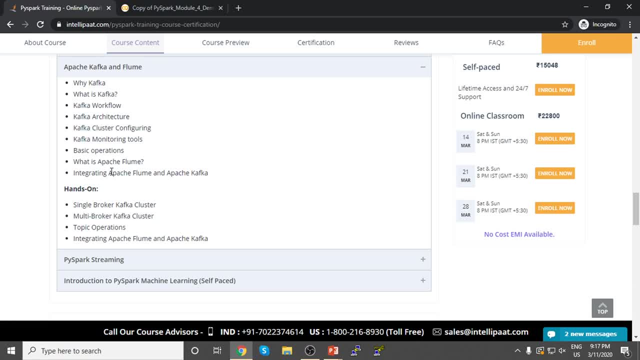 Flume. basically, all of these things are for real-time analysis, which is very important in the big data field, as we discussed before, Then the velocity factor of it and PySpark streaming, which means, again, real-time. Streaming means real-time. 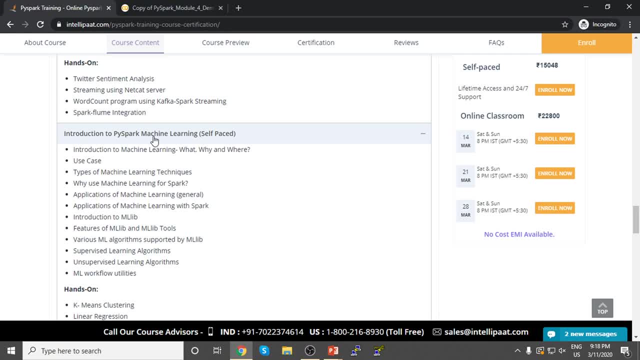 And the last part is which we provide a self-paced thing where you can develop and implement your projects at your own pace. Once you understand how to store and process big data using PySpark, you can obviously use the implement present in Python for the machine learning operations. 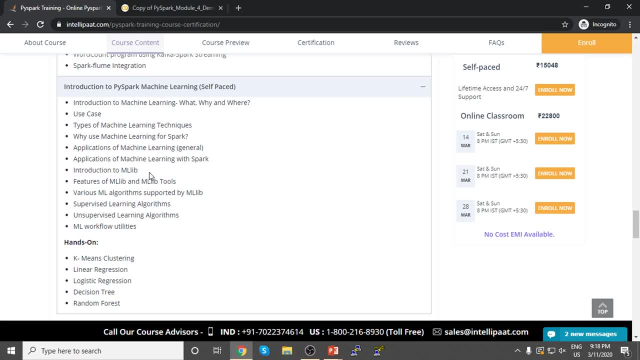 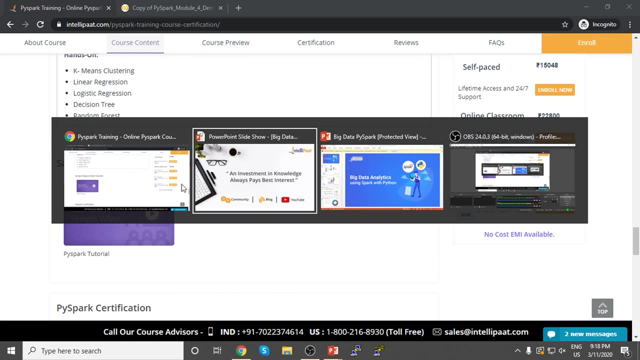 for Spark And you can also use data that you understand from Spark So that you can experiment with on your own and get better at understanding how big data works. So now that we know what course content is, that would be about it, So we've discussed that. 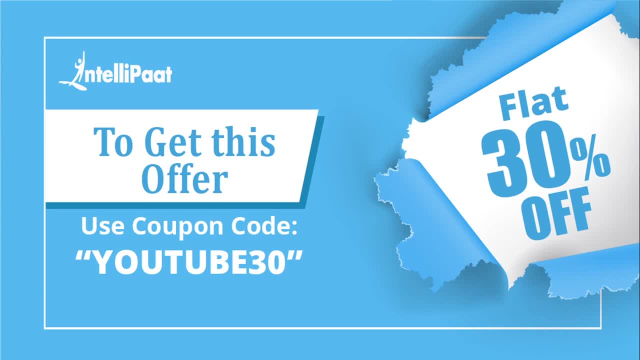 So, especially for the viewers that are watching us here today, we have a surprise for you. If you use the YouTube 30 coupon code right now on our website, you will get the course with a flat 30% discount. So be sure to avail this offer. 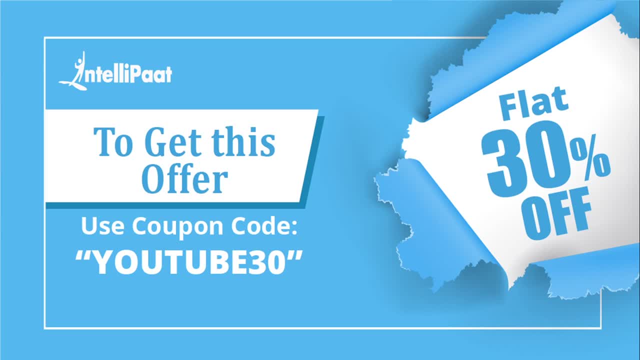 if you're looking to get into big data and Scala, Spark developing engineering, PySpark engineering, So use the coupon code YouTube30 and you'll get it for 30% off. So that would be it for this session, guys. Hope you enjoyed it. 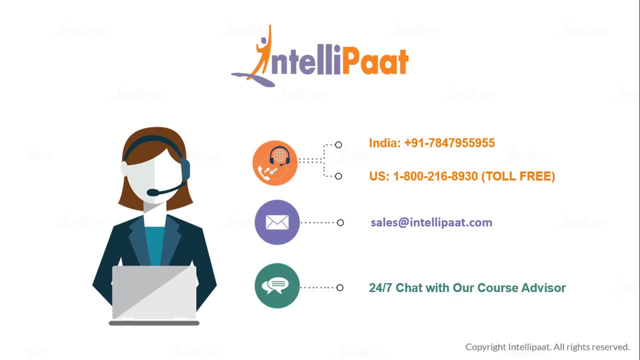 I'll leave some contact details here for you to contact us if you have any doubts or queries, if you want to understand the course content any better, if you want to understand our services any better. So thank you for attending the session, guys. 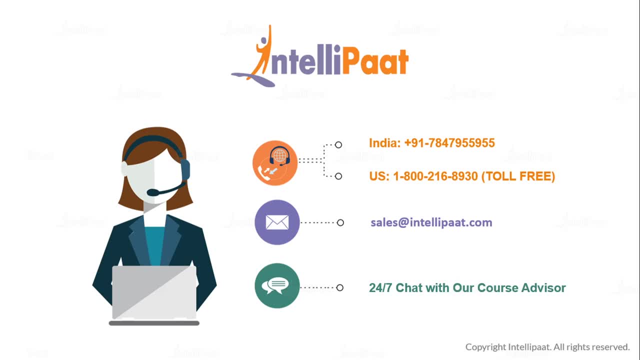 That'll be it from us. Have a great day, Thank you, Thank you.